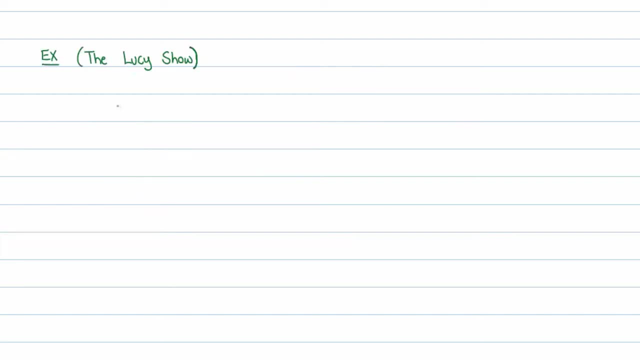 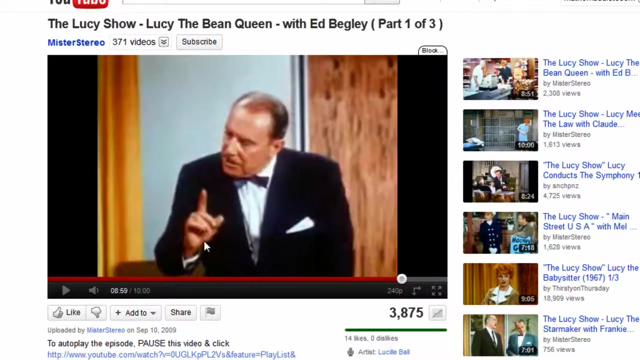 just problem-solving skills. now, our very first example here, and normally I wouldn't start with an example, I'd actually start with a concept, but I I want to build the concept from an example, and this involves a video clip from the Lucy ball show, or actually the Lucy show. here we go. I want you to 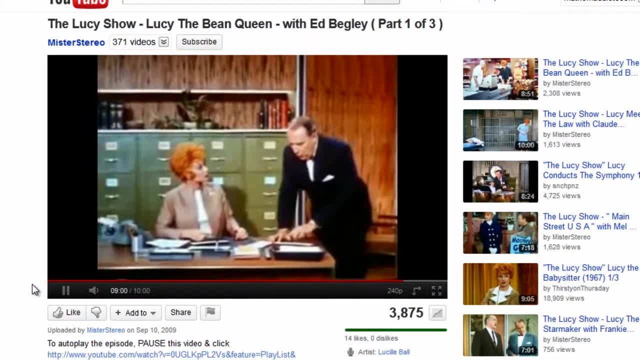 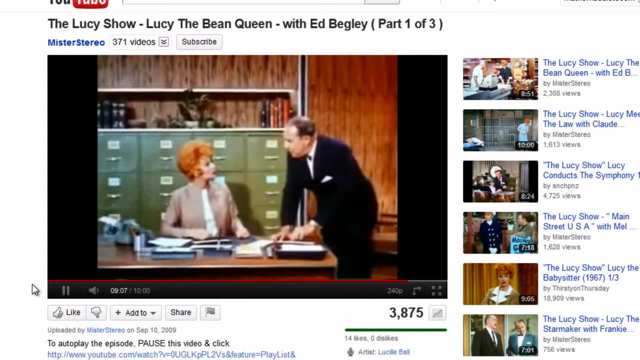 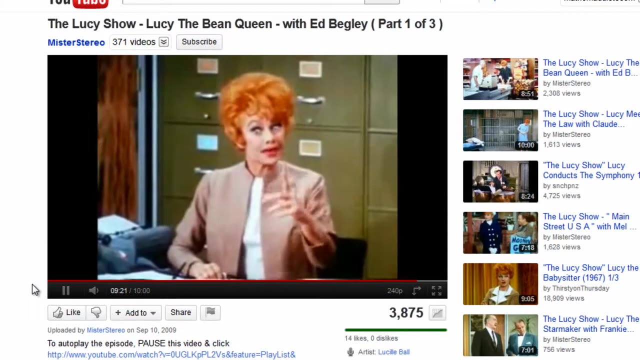 listen to this just for a moment. if you put one penny in the bank today, two pennies the next day, then for the following day, and keep doubling the amount each day, you would have enough money to buy your furniture in 19 days. you're kidding, you mean, if I doubled a penny 19 times, I'd have $1,500. you would. 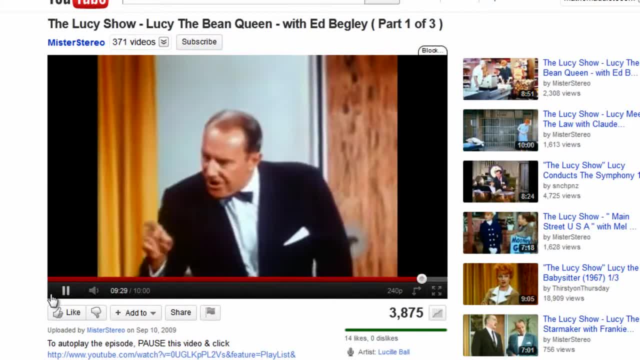 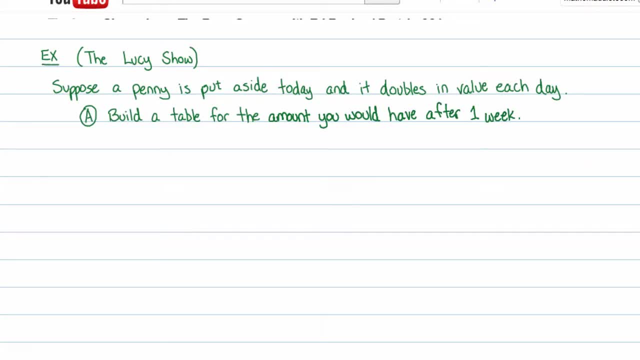 have more than $1,500 now. you just think about that. okay, so let's actually think about that. so that problem is essentially saying: suppose a penny is put aside today, okay, so let's actually think about that. so that problem is essentially saying: suppose a penny is put aside today. 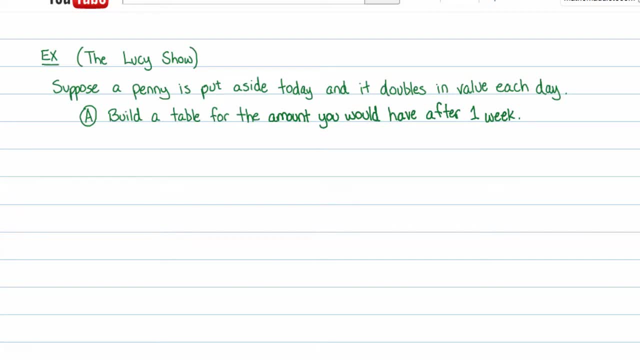 invested or put into the bank and it doubles in value each day. I mean in that problem actually he's saying you put a penny aside today, you put two pennies aside tomorrow, you put four pennies aside the next day. so he's kind of forcing her to put her money down each day. but I'm saying, suppose you could. 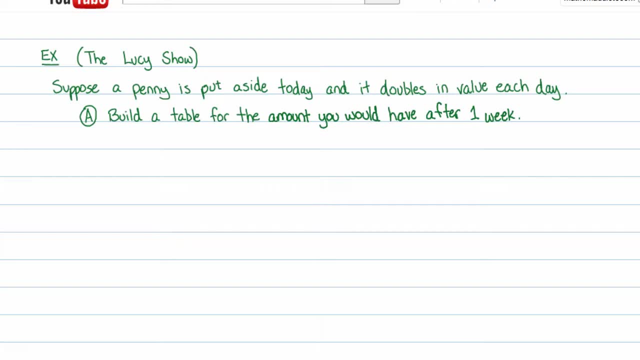 just drop a penny and somebody who's willing to double it every day. let's build a table for the amount we would have after one week. so what I'm gonna do is use function notation here. I'll let D equal the number of days that have passed and I'll 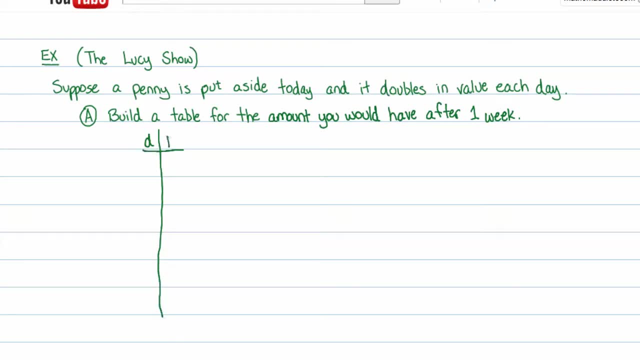 let I'll let P be the number of pennies we have at that number of days. so on the 0th day, in other words the initial day, and that's that's generally what we we start with when we're talking about doing something. today we just we talked. 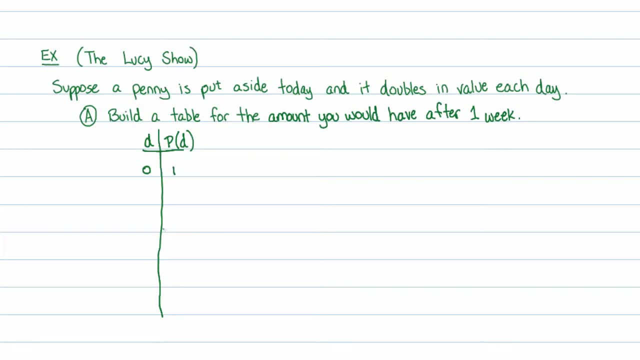 about the 0th day, we we have one penny, but tomorrow it's gonna double right. tomorrow, the end beginning of day one, one day ahead now, we're gonna have double that or two pennies, and the next day we're gonna have double that, two or four pennies. now, 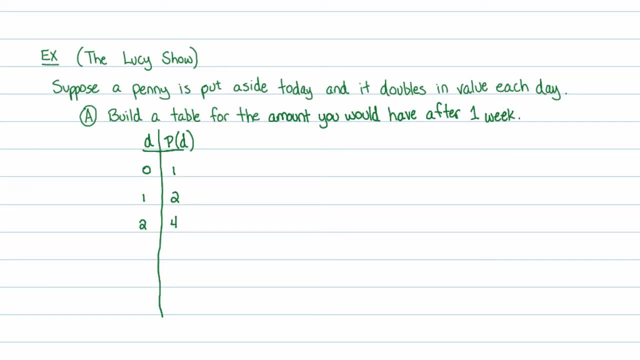 how did I get that? for? well, let's see, let's go back and see how I got the two, the two I got from saying, well, I'm gonna double what that last number was, which was one, this four I got, because I'm doubling what that last number was. 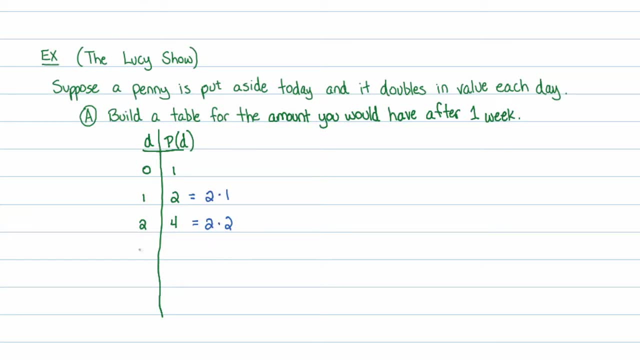 which was two. the third day: I'm gonna double the last day. well, let's see here. the last day: I'm gonna double what the last day was. last day was four. oh, but wait, let me write this as two times four is just two times two, so that's two times. 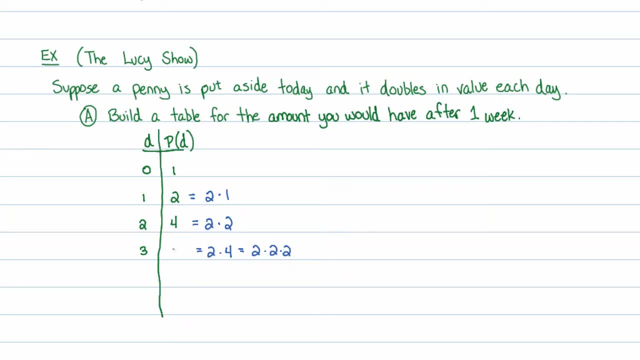 two times two. now you might be asking why I would write it like that. I'll show you in a moment. but it's just double four, which is eight. four days later we're gonna double up on that eight, and everybody knows a double up of eight is. 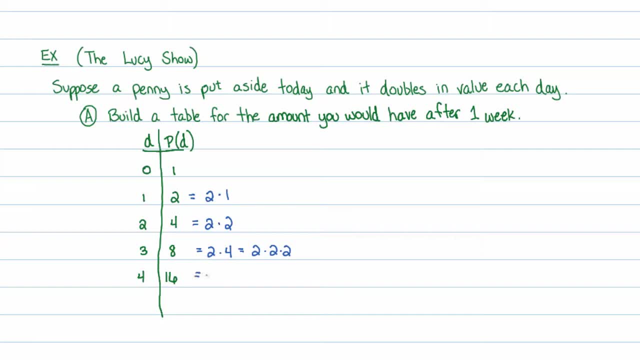 sixteen. but let's see how we would have done that mathematically would have doubled up on that eight. but again, eight is just two times two times two. so that'd be two times two times two times two. well, this gets kind of long-winded writing out like this, so let me use exponential notation. that's two to the. 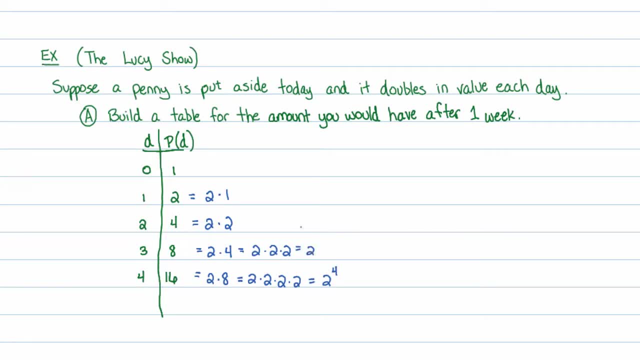 fourth power and this one back here was two to the. actually let me even write this with a red four there. this is two to the third power and this is just two to the second power right, and actually this one right here is two to the first power right. two is just to the first. 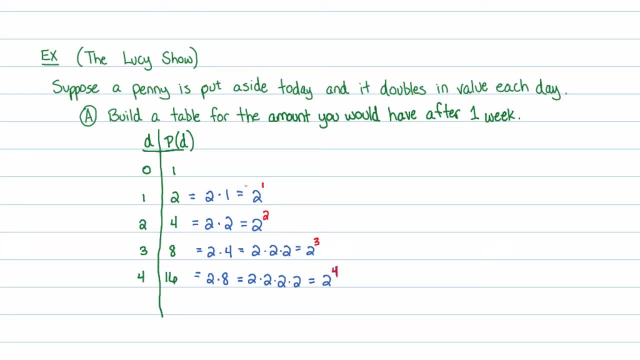 power. and you think: well geez, there's a pattern going on right. on day one, we have two to the first pennies. day two, we have to the second pennies. day three, we have two to the third pennies. day four, we have two to the fourth pennies. but 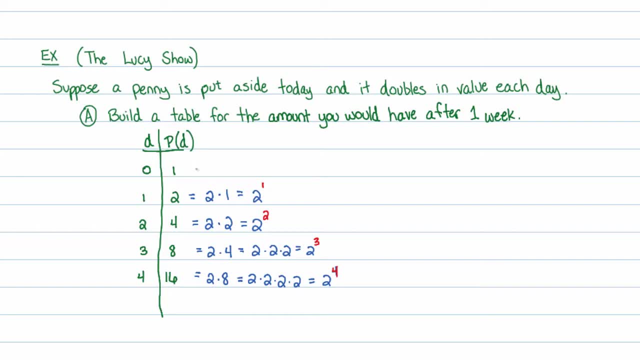 some people would argue that day one or day zero. I'm sorry doesn't work out, but it actually does because, remember, two to the zeroth is equal to one. any number to the zeroth power, as long as it's not zero, is equal to one. so that must mean that five days later we'll have two to 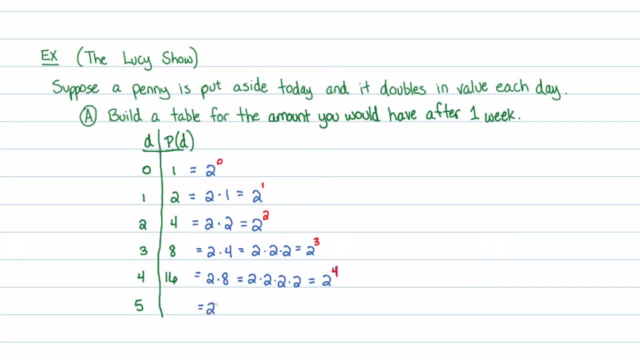 the fifth pennies, just following the pattern that we've just started to develop to the fifth. fifth is 32, which does work out, so I'll just write that in here: six days and seven days later. I know you might not be able to see the seven, it might be off your screen, but six days later we have 64, seven days. 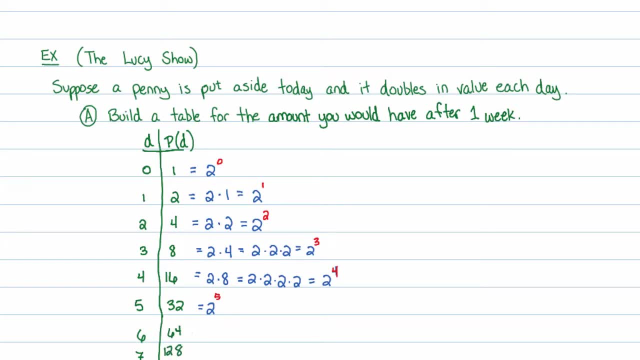 later we have 128 and, by the way, 64 is two to the sixth and 128, if I can catch up to myself, it's 2 to the seventh. so this is an interesting situation. it turns out that our outputs, it turns out that our outputs- 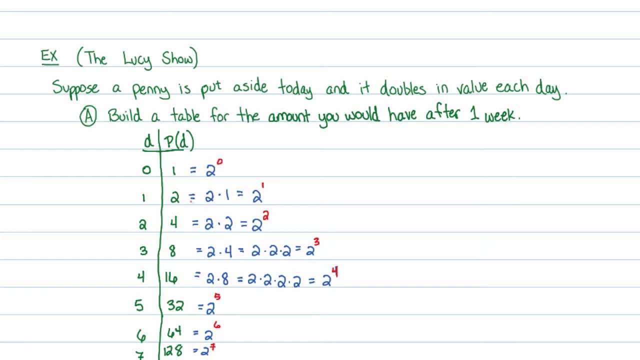 depend on how many times we have to play each of these very important numbers. so there's an interesting situation: turns out that our outputs determine how many- and these are done with your output- how many times we have to play each of these very important numbers depend on an exponent, the value of an exponent, and this gives us an idea for a new kind of 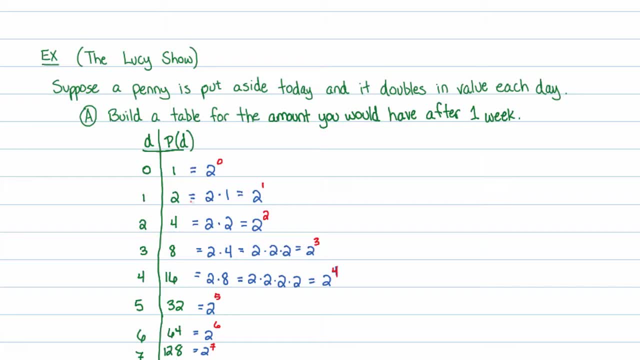 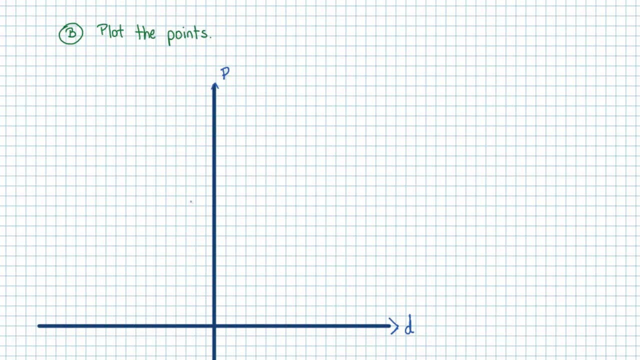 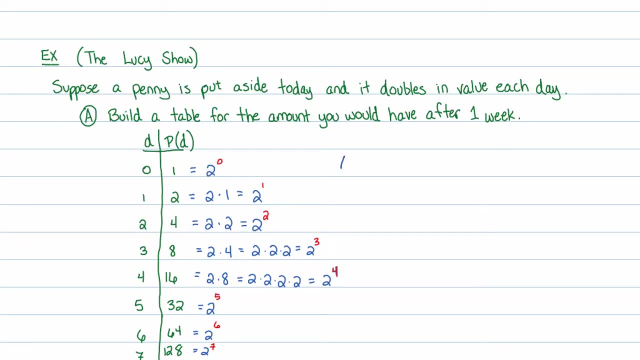 function, one that's called an exponential function. now, before I get into really the guts of an exponential function, let's plot these points back here, these ones that we've listed out. these ordered pairs can be listed as 0 comma 1, 1 comma 2, 2 comma 4, and so on. 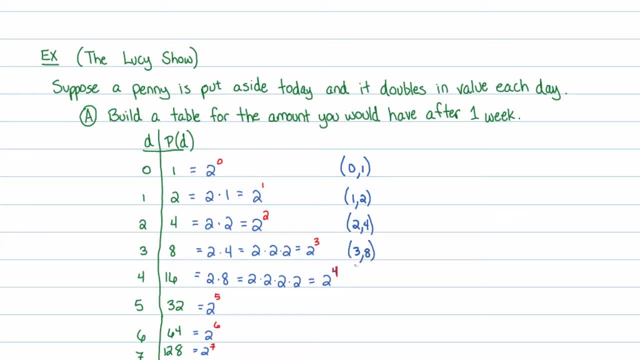 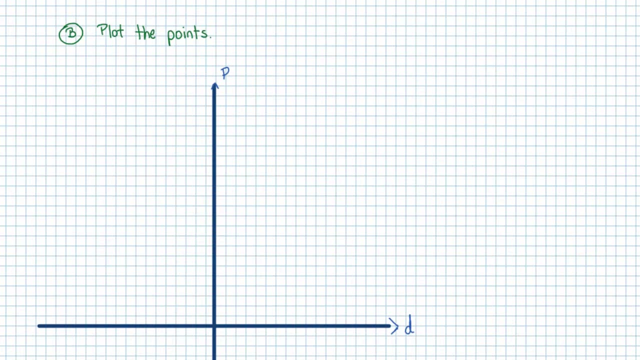 and so forth, right, so I'm not going to write them all out, but you get the idea: dot dot dot. so let's go ahead and plot those points, and I'll use a pretty decent color here to do this. let me change colors. so 0 comma 1 was our first one, so I'm going to plot that. 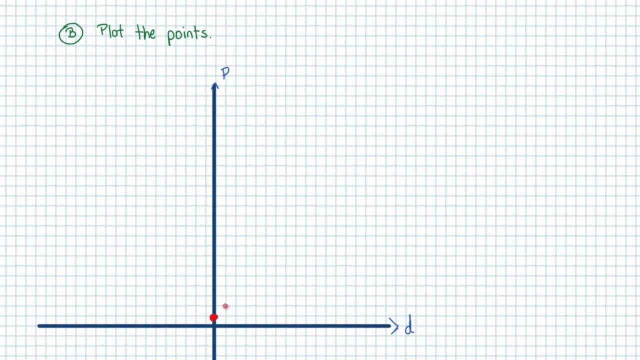 right here. and then 1 comma 2, it's right there. 2 comma 4, so 1, 2, 3, 4, right there, let's see. so 3 comma 8, that's 4, 5, 6, 7, 8. we can already see. it's not a line, right, let's see. so that's 1, 2, 3, 4 comma 16. so let's. 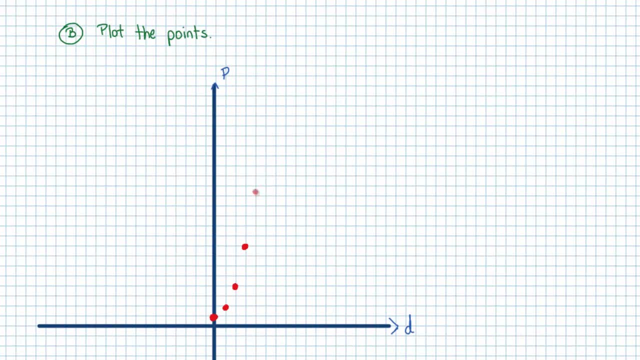 see, that's 8, 9, 10, 11, 12, 13, 14, 15, 16. you can see what's happening. it's really climbing up there, and then I'll see if I could do 5 comma 32 on here. and there we have it, in fact let. 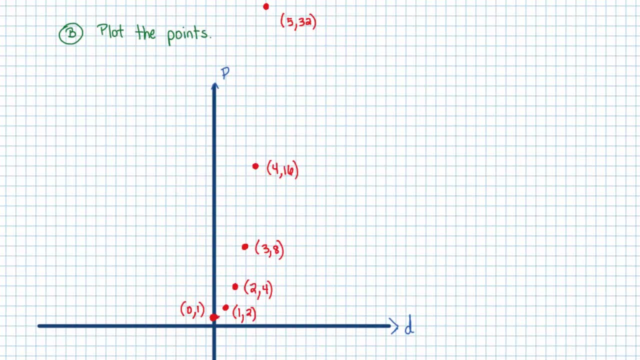 me label these and then I'll connect them up with a nice smooth curve. and this smooth curve, if you notice it's increasing faster and faster as time goes on, and that's a very good characteristic, a very good way to know that you're dealing with an exponential function. 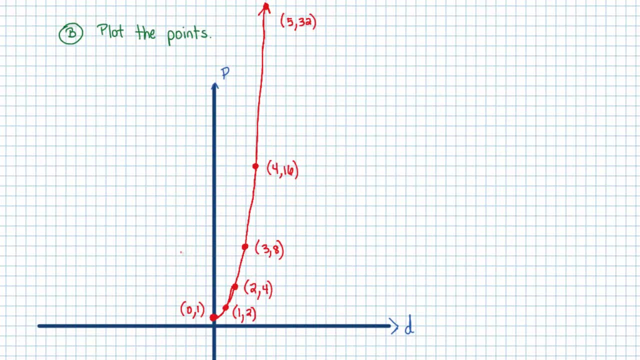 is that it grows well exponentially. that's why they call them exponential functions. it's a basic look of one. now we're missing part of the graph. actually, this graph, to be very honest with you, continues on this way as well, but we'll talk about that more in a different. 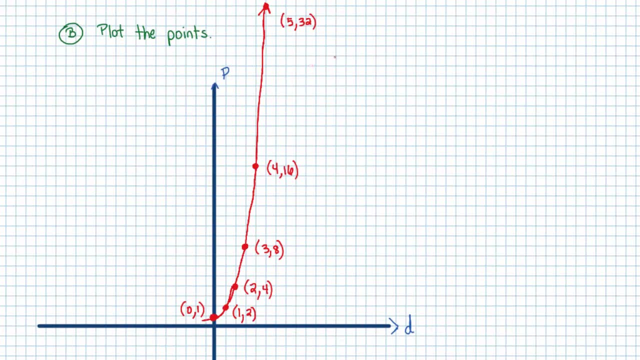 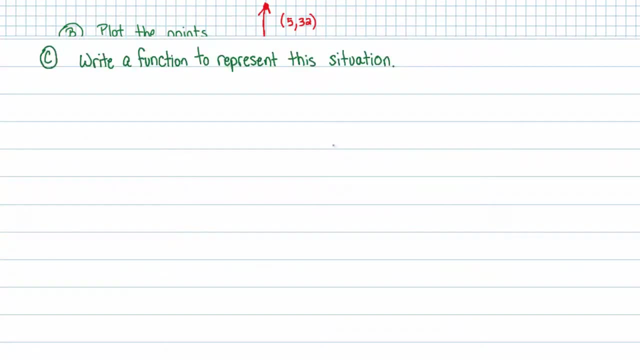 lecture. so I just want to get the basic idea of what the kind of the overall look of it is as time goes on, as it ticks on and on and on. now here comes the meat and potatoes of this problem. we want to write a function that represents 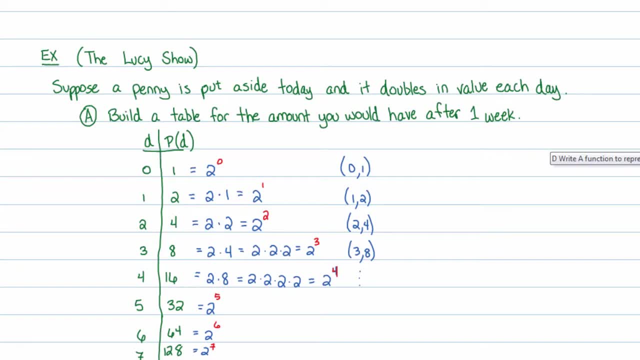 the situation now. here is our table of values and you kind of tell that it's. the pattern is, whatever we plug in for D, the output that will be to that power. but I plug in two. our function won. the output will be to the first power. if I plug in to, the output will be to the second power if I plug in 15. 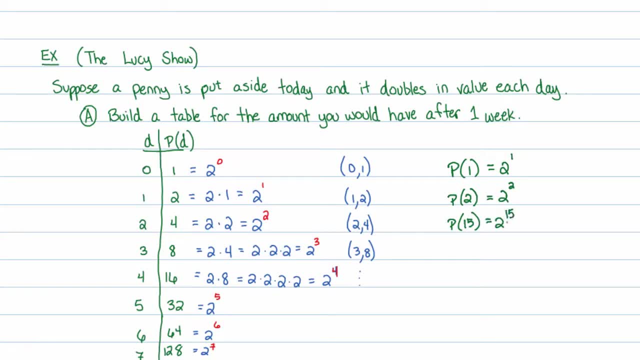 to say the output will be the 2 to the second power. if I plug in 15, 10, let's say, then the output should be 2 to the 15th power. now, if i plug in a variable like the number of days that have passed, the output should be 2 to the. well, follow the pattern here: the d power. so it turns. 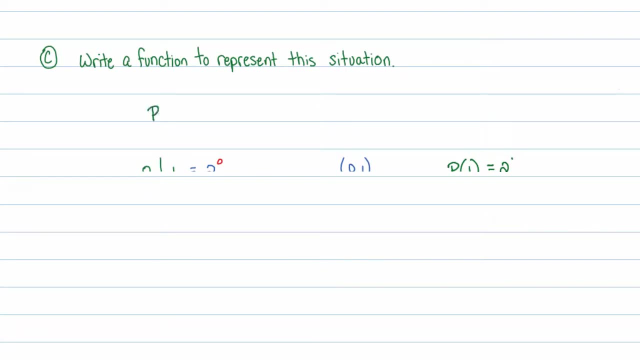 out that our function is just p of d. number of pennies at day d is equal to 2 to the d power. now remember in that problem, uh, that the video from the lucy show there. he said that after 19 days lucy would have enough money to buy her couch and she was pretty impressed with that. 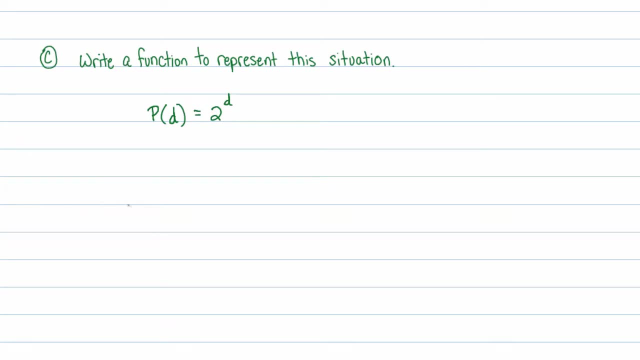 well, let's see actually how much somebody would have, let's say, after a month, and in this scenario, let's consider, uh, that to be 30 days. it doesn't really matter, you could say 31 days if you want, you'll just have more money, you. 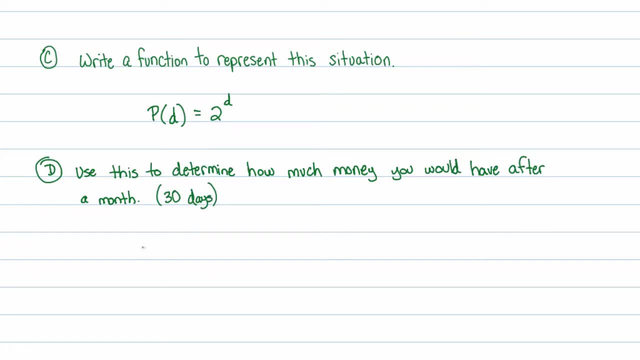 so this means that p is going to be evaluated at 30. we're going to let d equal 30, so this is the amount of pennies we're going to have: 2 to the 30th. well, you might not feel as though that's. 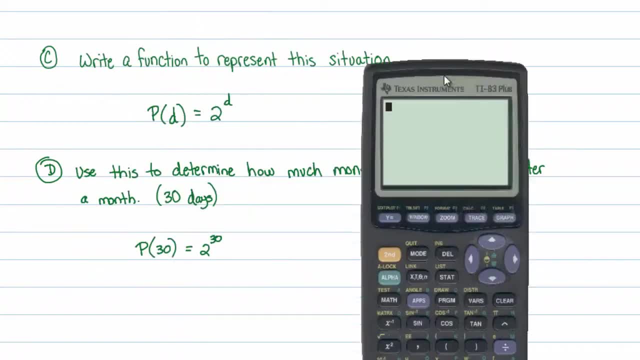 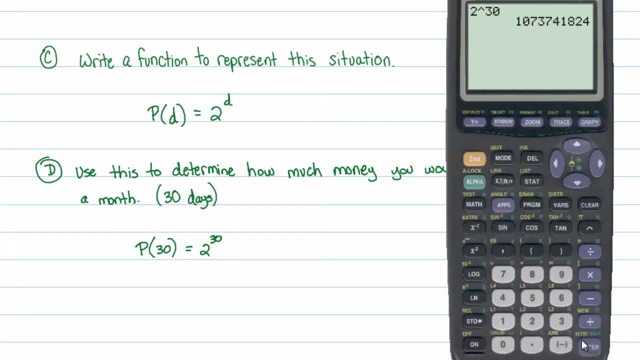 a lot, but if you bring up a calculator and just type in 2 raised to the 30th power, you'll find out very quickly that that is quite a bit of pennies. remember, this is pennies, so this is going to be 10737. uh, what is it? 41824, 41824- now, that's in pennies. i'm going to put a decimal point here. 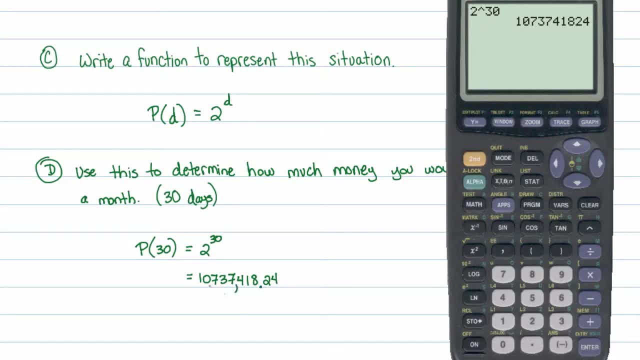 to make it dollars. so let me put a comma and a comma, oh, that's just 10 million dollars, almost 11 million dollars, starting from a penny doubling every day for a month, just 30 days. that's about it for today's video. i hope you enjoyed it and i'll see you in the next one. 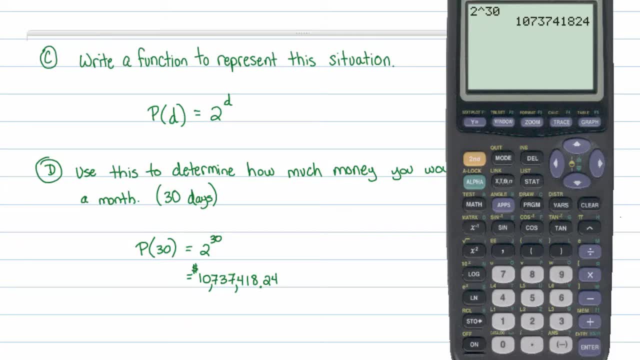 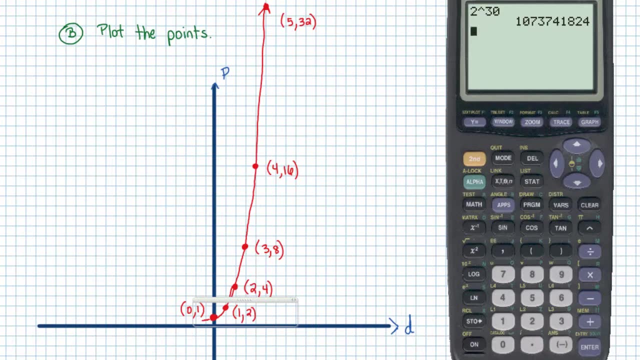 bye, bye, bye, bye, bye, bye- pretty ridiculous. but if you think about what this graph shows, it shows that the amount of money we have can grows continually. after five days, it's shot up this much all the way up to here and it's just going to grow faster and faster as time goes on. so this is the behavior of what's. 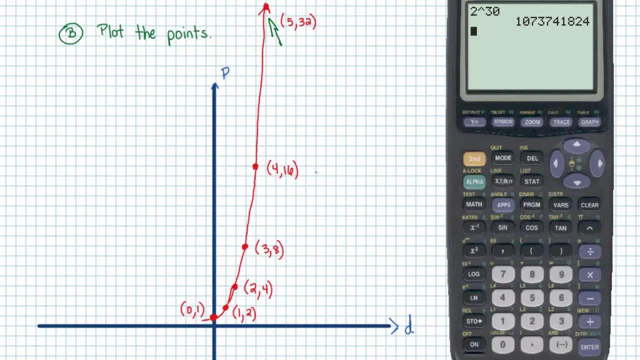 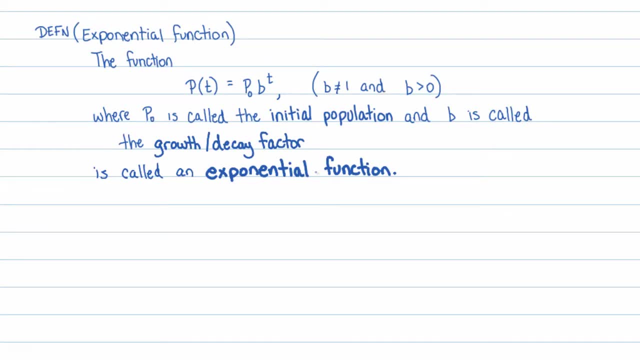 called well, this is called exponential behavior. the official definition of an exponential function goes like this: the function p of t. now, it's very important to realize here that there's only one. well, there are two unknowns, but there's one independent variable, one dependent variable. the independent variable is what we're plugging in, right, so we're plugging in t. 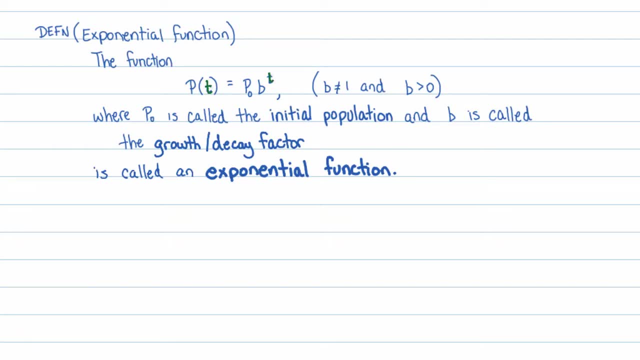 notice where that independent variable is in this equation: it's in an exponent. that's a great indicator that you're dealing with an exponential function. you're dealing with an exponential function is that your unknown is in the exponent. that's the only time you call something. an exponential function is when your unknown is in the exponent. okay, so this function p of t- 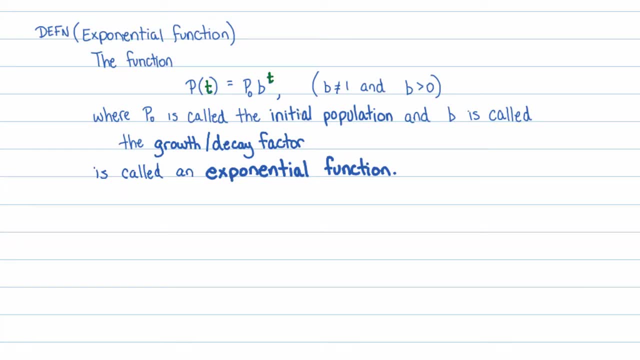 equals p naught, let's pronounce p naught or p sub zero. i'll just write this in as p quote unquote: p naught, p naught times b to the t power, where p? naught is called the initial population and b is called the growth or the decay factor. this is called an exponential. 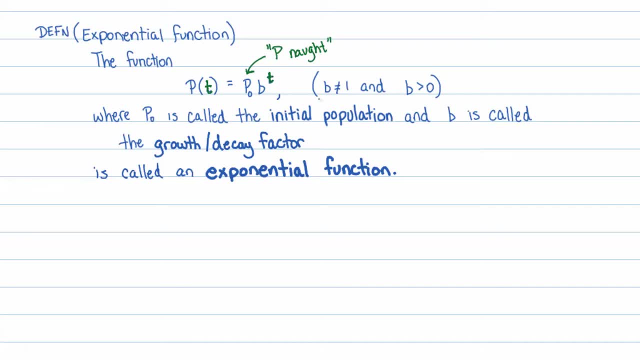 function. now let's a few of these things need descriptions before i go any further. one thing is that you notice is in parentheses there i have- that b cannot. b cannot equal one the reason why b cannot equal one. well, if it did, you'd have something like this. let's just: 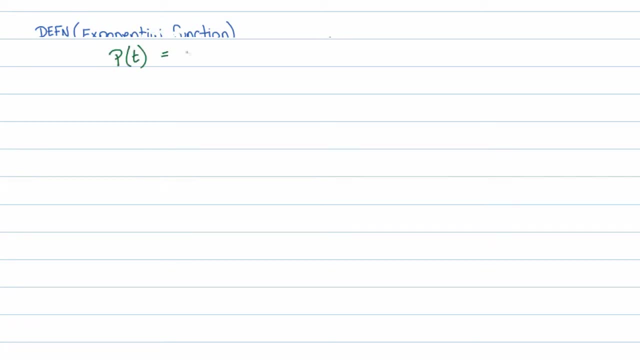 make a exponential function up. let's say we just had some initial population, let's say two, and let's say our base was one. well then, 1, 2, the power is just still one. so this is the same thing as just saying 2 times 1, or in other words 2. this doesn't grow, this is just p of t equals 2. this is 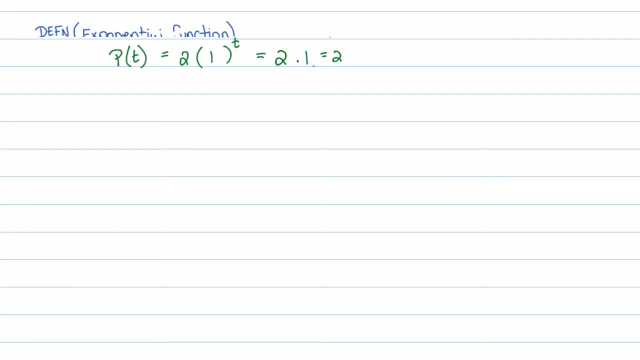 there's nothing changing with this. doesn't matter what i plug in for t, this is always going to be 2. so that's a little bit silly. you can't, we kind of say that you can't let b equal 1, because well, that's not exponential, it's not doing anything. the other condition: that b has to be positive. 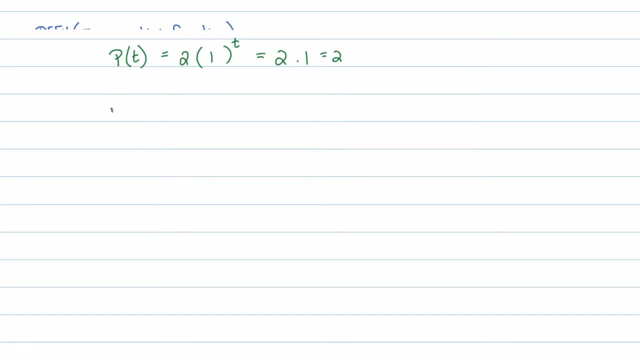 positive is sort of a tricky condition. I'll tell you why. it's true, though, Let's suppose for a second that we allow b to be negative. So let's just say we have the same initial population, but we choose our base for our exponential part to be negative. Well that's. 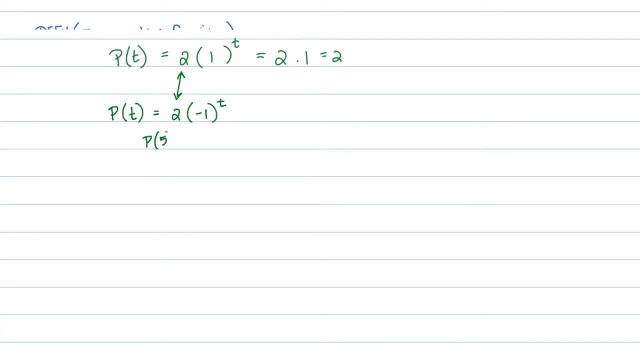 fine if p is like 5.. If p is 5, then you have 2 times negative 1 to the 5th power. Well, negative 1 to the 5th power is just a negative 1, which is going to be a negative 2 altogether. 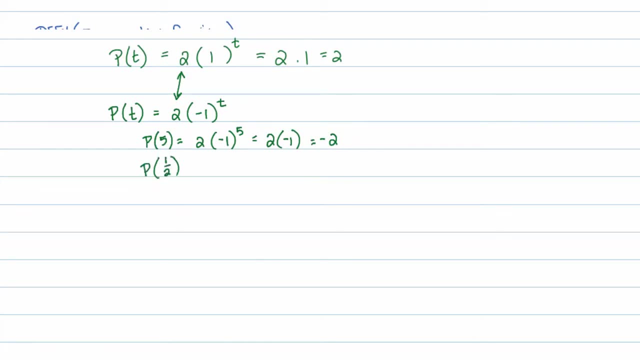 The issue happens when you do like things like p of 1 half. That would be 2 times negative 1 to the 1 half power, and remember, 1 half is a square root, so that's 2 times the square root of negative 1 and we've got an issue right. That right there tells us that we can't. 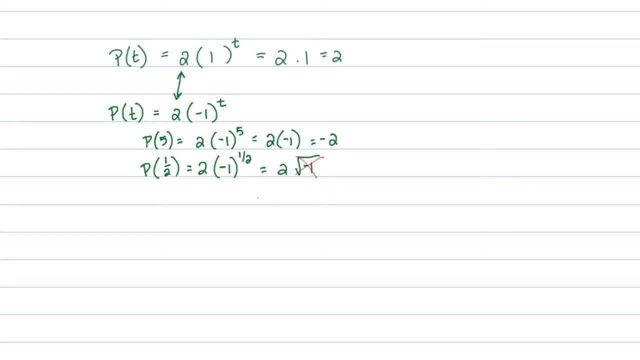 go any further, Cross that out. That's non-real. So that's why we kind of require that we let b be positive. And again, the first reason was why we require b to not equal 1.. Now let's explain the other thing here, P naught is called the initial population. I'd like you. 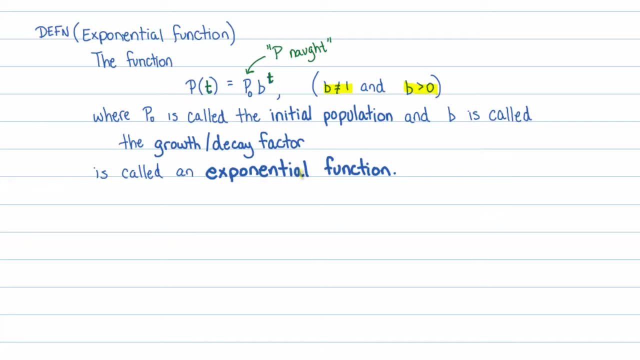 to really know why it's called the initial population. It's very easy to understand why it's called the initial population if you take it mathematically. If you let p be 0, t is just time. It stands for days, weeks, years, hours, seconds, whatever it is. If 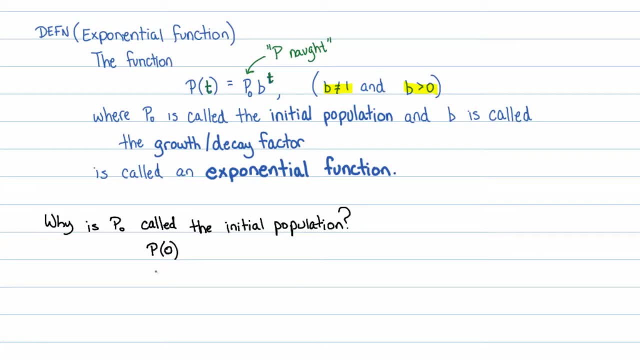 you let t equal 0,, in other words, time 0,. right now, the initial time. Let's see what this turns into. It turns into p naught: b to the 0th power, But b to the 0th any number. 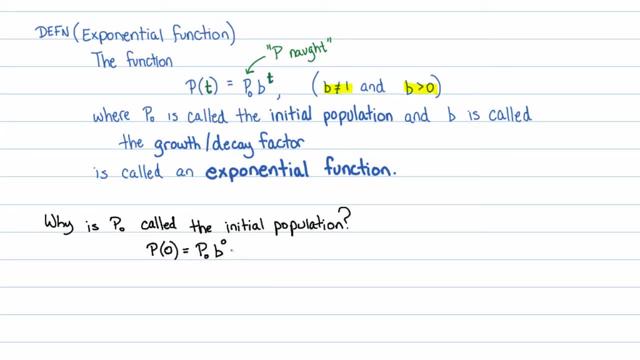 to the 0th power. as long as that number is non-zero, is going to be 1.. So that's just the same thing as p naught times 1.. Well, p naught times 1 is still just p naught, So 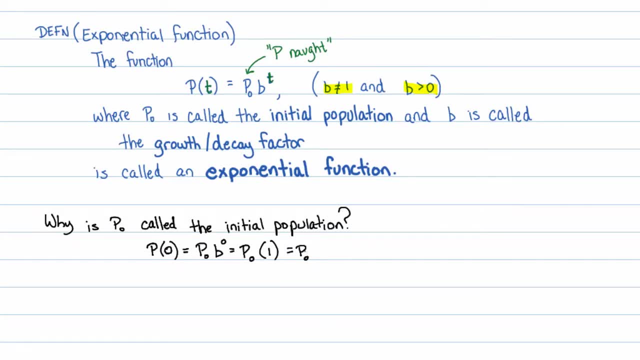 notice that p of 0 is equal to p naught. In other words, p naught is the value of the function at time 0. That's why I call it the initial population. So we now have seen why this is called the initial population, B being called the growth or decay factor. that actually 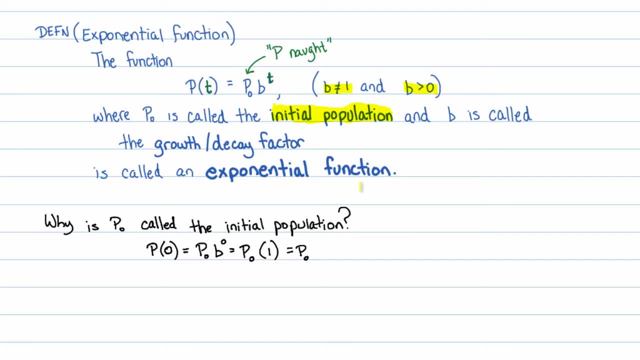 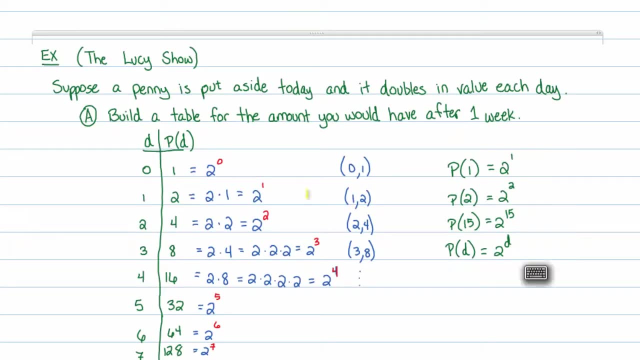 determines how quickly things are growing or decaying. So if we go back to our example- we had a few moments ago this one right here with the Lucy Ball show- Notice that the base for our function. in fact, let me go to the function itself, The 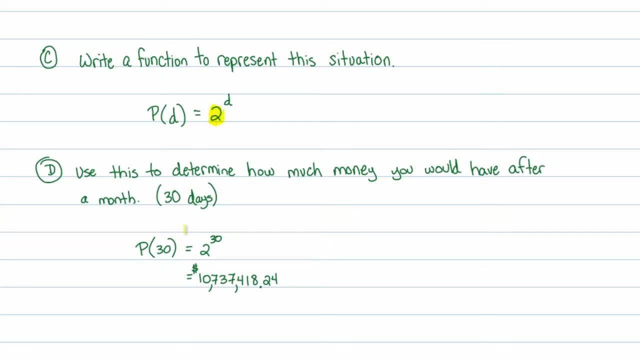 base for our function is 2.. It's because it's doubling every day. So that tells us. I mean, when I read that p of d is equal to 2 to the d power, I immediately think, oh, the base of the exponent is 2, that means it's doubling. If the base of the exponent was: 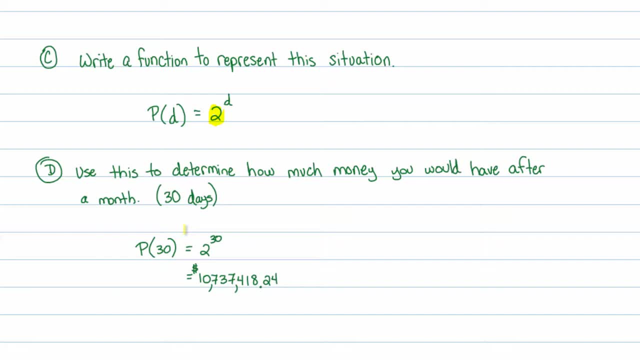 3,, it means that it would be tripling. If the base of the exponent was 4, that means mean it'd be quadrupling, and so on and so forth. it's a very nice kind of organic way to feel that out. by the way, this is an exponential function format, but if you really want to match this, 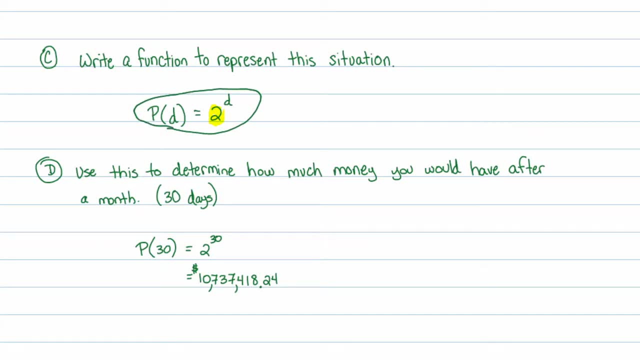 function here up with our definition, then we need to put the initial population down. well, if you read the problem- and that's by the way, i used the letter p not because of pennies, even though i said it was for the fact that we were dealing with pennies. i use the letter p because 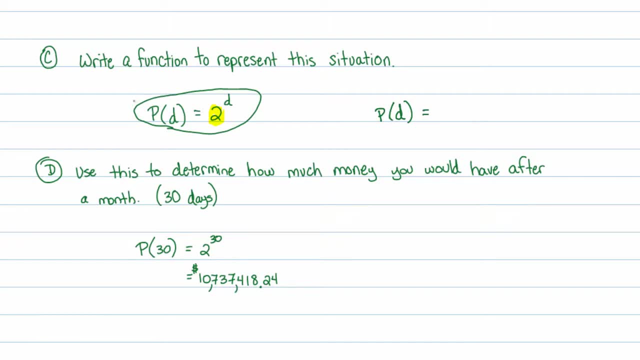 p i always use with population models and i consider an amount of money in my bank a population of money in my bank anyway. um, this can be written in that form of p, not times b to the t power. if you think about the initial population, initially we had one penny and then it doubled every day. 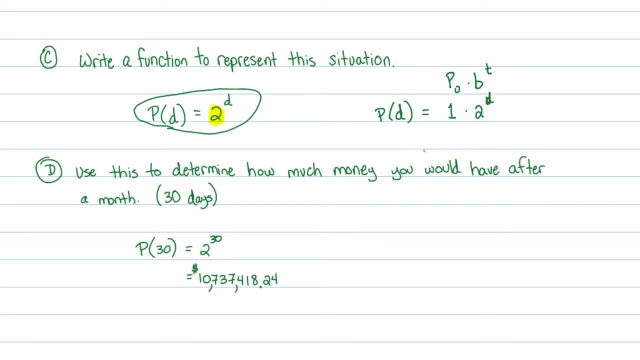 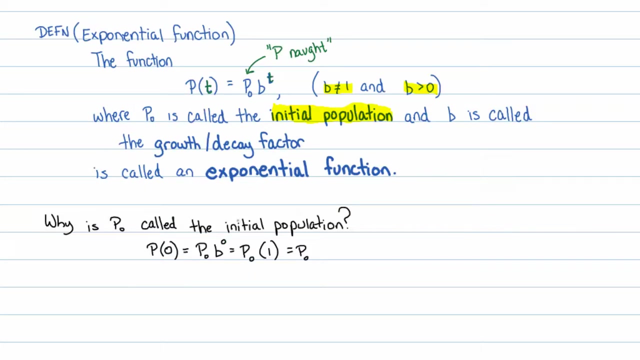 there you go. that's the. i mean, that's the same thing, so but but often we don't write the one, so this would just be: p of d is equal to to the d power. now, i don't expect you to be an expert right now, but at least you kind of understand the bits and pieces of this. i'll refer to a lot of these as 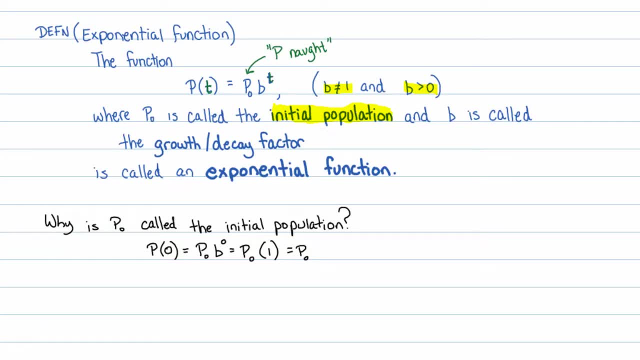 we go along. there's more to the growth and decay factors than what i'm saying right now. but uh, we'll get into that in a moment. i don't want to, or actually in a few minutes, but i'm going to go back to the future lecture. i don't want to over confuse you right now. just know that, whatever this, 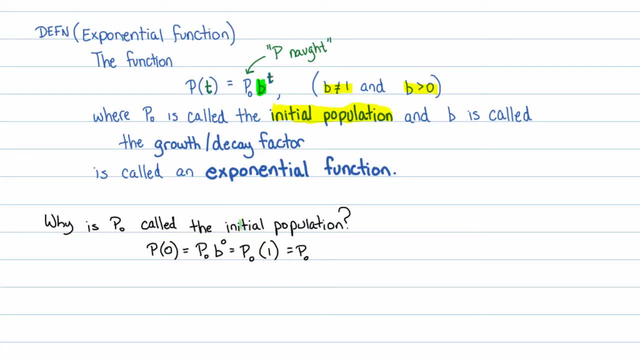 value of b is. whatever that value b is, it controls how quickly things are growing or how quickly they're decaying. and notice, i haven't given you a decay example because they're a little more in- involved, i guess, is a good word for it. they're a little more involved and i don't want to get too. 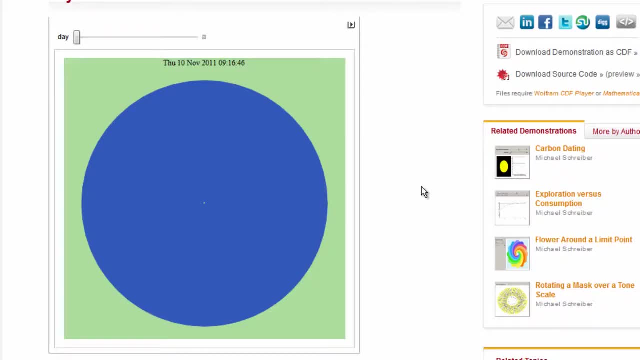 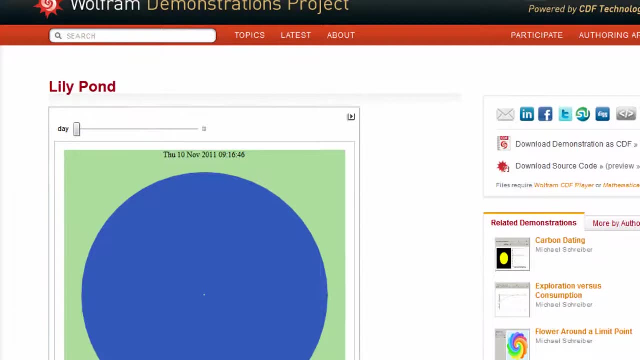 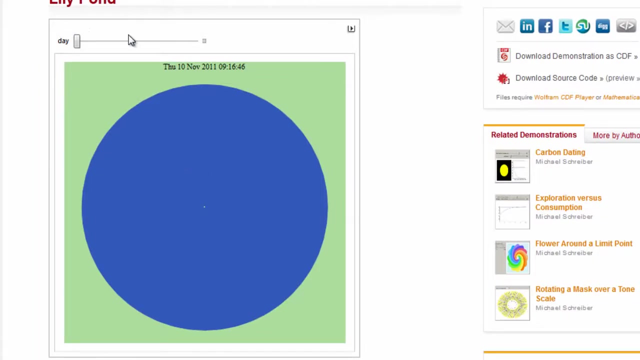 involved at this point. now i want to give you another kind of visual of exponential growth. this is a lily pond example from wolfram demonstrations project, and what i'm going to do is control the number of days have passed and let me describe the situation you have. 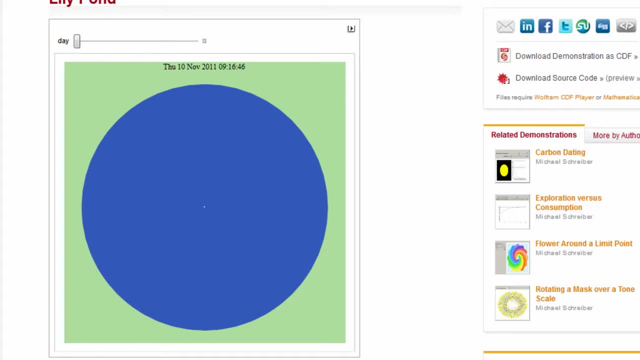 a water hyacinth. a water hyacinth is just uh, basically a water, uh, like a like a grass. it's not really a grass, but it's. it's a type of weed that's in water, and it doubles in population every twelve days. 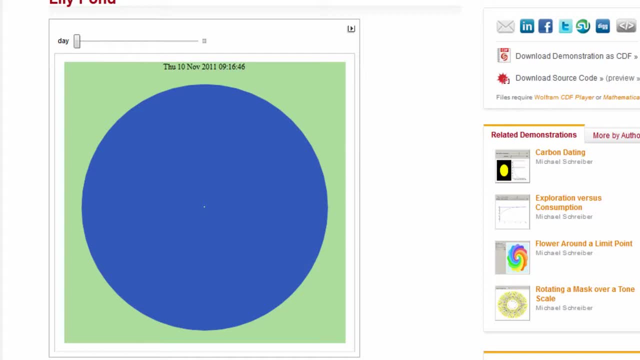 so every twelve days. if you started with one, twelve days later you'll have two, and twelve days after that it'll double that two and become four, and twelve days after that it doubles and becomes eight right, and so on and so forth. so what i want to do, 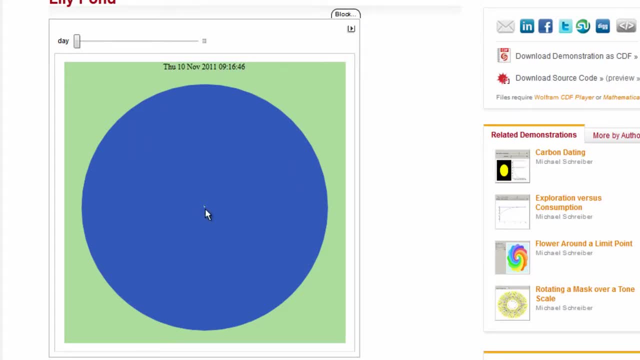 is. show you. this is a big pond of water. there's a little green dot in the center. that's one water hyacinth right there, and i'm going to let time go on. so it's thursday, november tenth two thousand eleven. i'm going to see how long it takes to fill up this pond. 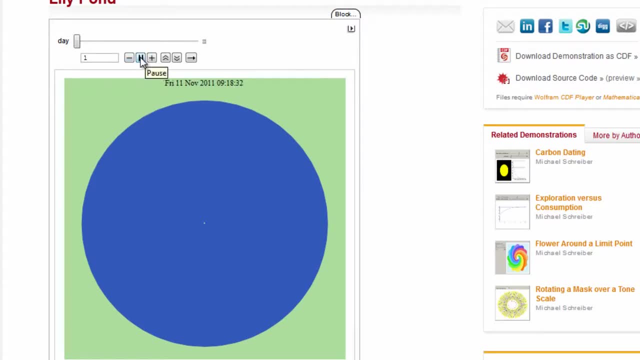 so here we go. i'm just going to hit play on this. now notice the days are just jamming forward. i'll slow them down a little bit. see, we're in december, january. you don't see a lot of. i mean, it doesn't look like it's changing, but there's, it's actually been doubling. 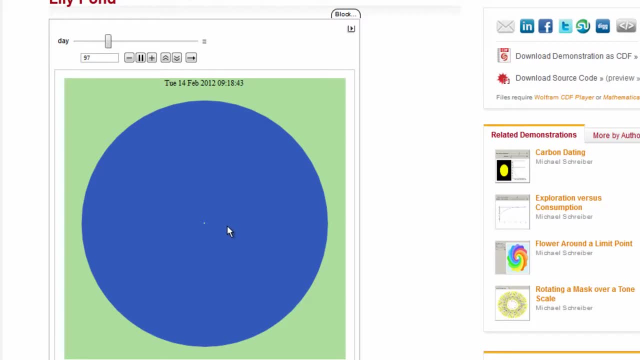 it's just very slow. you'll see this point get bigger and bigger. actually it stopped, so hold on. okay, so we're back to moving forward and you see now that that's doubled by twice, that the dot is actually doing something in here. okay, we pause again for a moment. 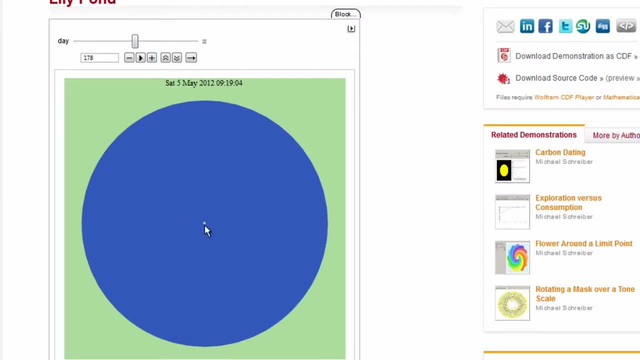 I just want to point out that this dots a little bit bigger because it's been doubling. I mean there might not be a lot of water hyacinth here. we're at day 178 right now, but as we move forward you'll see it does actually once you start. 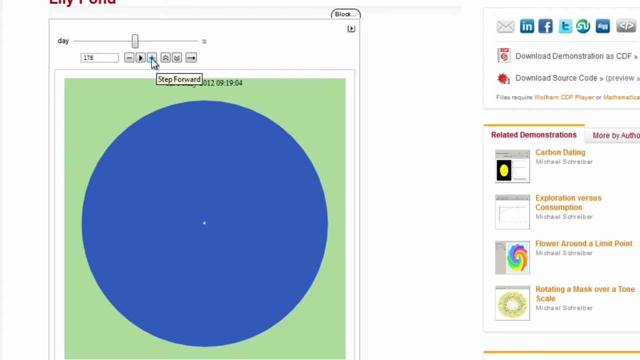 getting just a little heavier population. doubling really makes a difference, so let's go ahead and continue forward. you can see that it's growing and growing. right now you can really see the doubling. we're at 250 days. I mean it's, it's. the population is basically exploding. so it took a very long time. 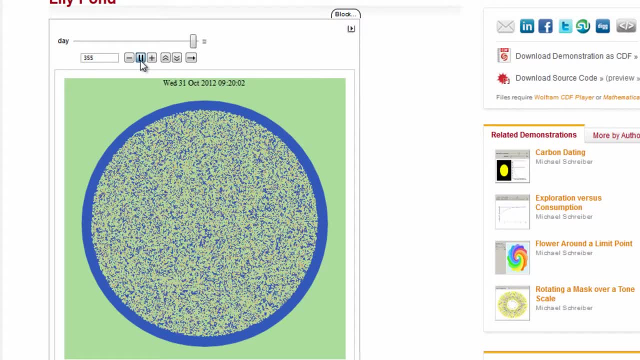 initially, but then, once you get some growth going on there, let me pause it right now. 357 days once. once the growth starts going, it just boom, and that's generally how exponential functions work is that it may seem slow at first, but at after a few steps it just starts blowing up and I really like 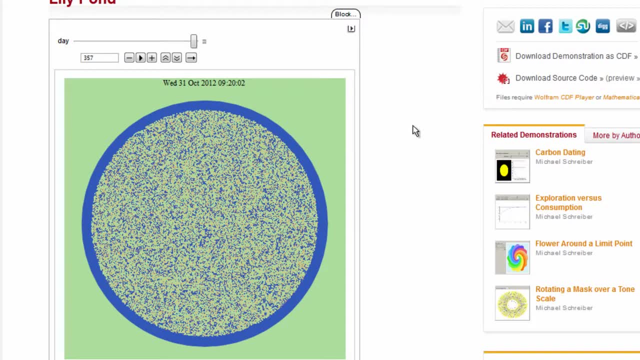 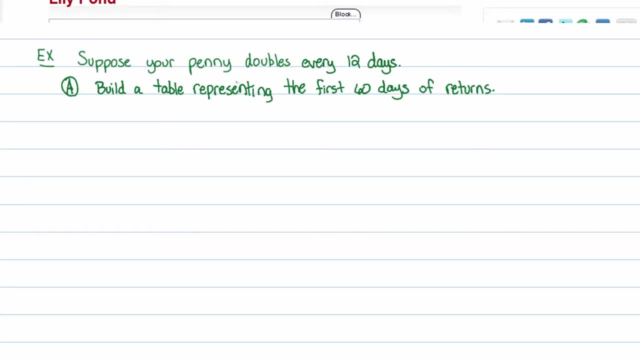 this example actually. so let me use this example with our money example, so I'm gonna kind of mix the two. so let's suppose our penny doesn't double every day, but now doubles every 12 days. so, just like that water hyacinth example, we're gonna build a table right now and we're gonna start building a table right. 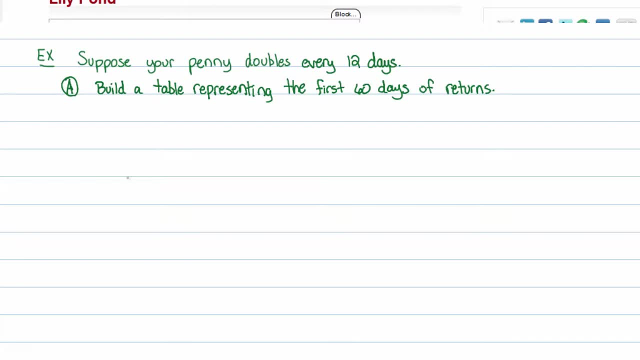 now we're gonna build a table with 60 days in it. I'm going to take them 12 days at a time, so I'll have the number of days that pass here. that'll be our input. that's what we get to control. we get the control how many days pass and depending. 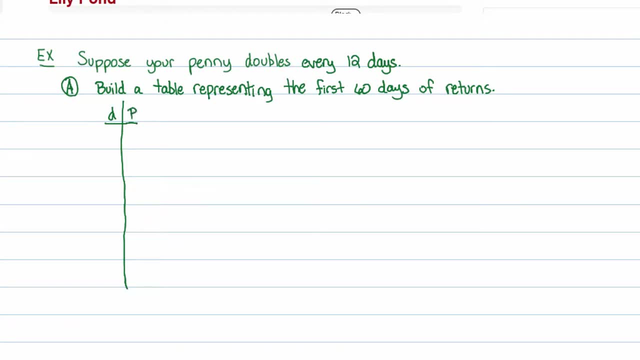 upon that number of days that have passed, we'll have a certain number pennies, so this is gonna be a new function. I'll still use the letter P for it, just because that's a letter I commonly use for functions, and I'll just worry about day 0, the initial day. 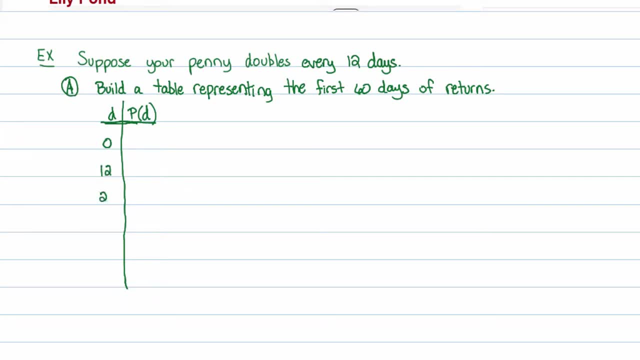 Then I'll worry about 12 days later, and then 12 days after that, and another 12 days after that, another 12 days after that and finally another 12 days after that. So that's the first 60 days divided up into segments of 12.. 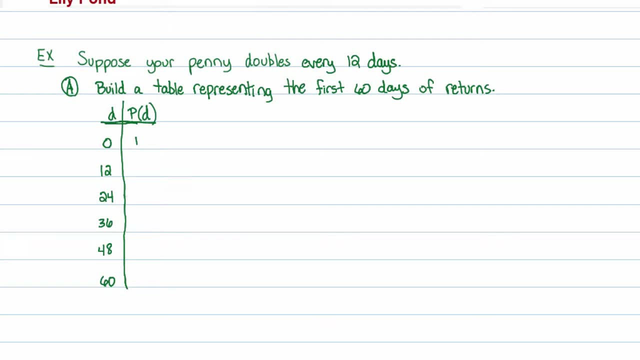 Initially, I only have one penny right, So that would be our 2 to the 0th, And then day 12, it doubles, so I'll have 2 pennies, And this is what's weird is that this is not 2 to the 12th, is it? 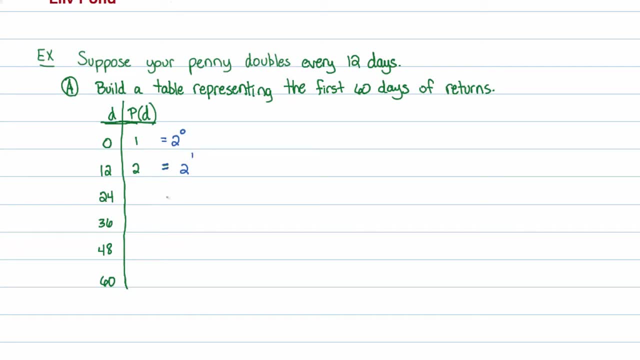 It's 2 to the 1st, so what the heck happened? Well, we'll find out 12 days later. it doubles to become 4, which is 2 to the 4th Or 2 to the 2nd. sorry, I didn't mean to say 2 to the 4th. 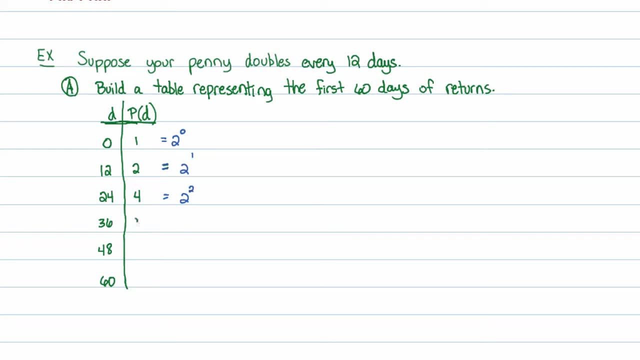 And then 12 days later it doubles again and becomes 8, which is 2 to the 3rd, And so on and so forth. But what's really important to ask is what happens? what if I don't want to know how much money I have at exactly a multiple of 12 days? 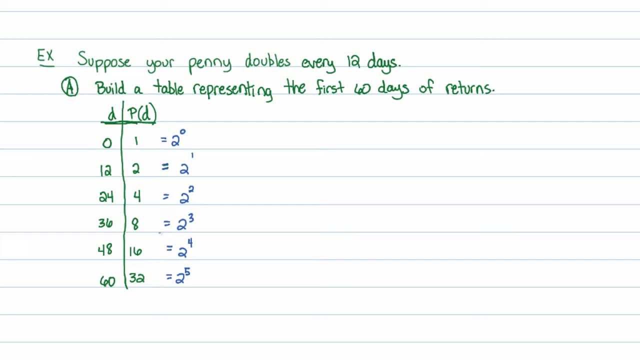 What if I want to know how much money I have after 13 days or 15 days or 21 days or 37 days? In that case, you're going to have to really kind of Just take a pattern from the beginning here. 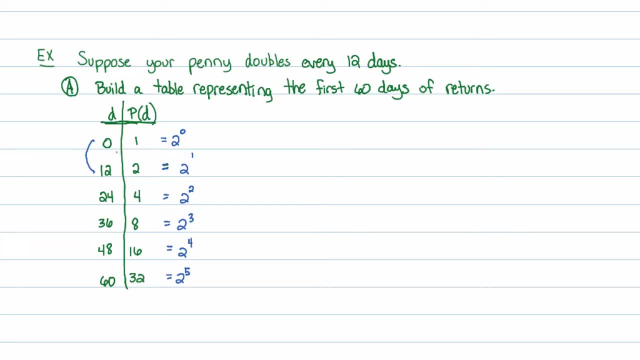 Try to develop some way of talking about these powers for the first 12 days first, so you can kind of see what's going on. Well, if we were at day 1.. So let me just put up a side table here. 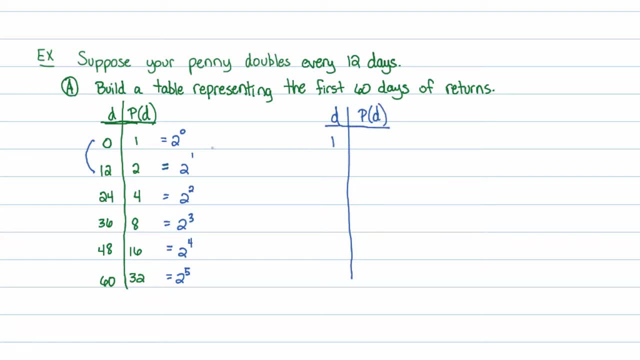 If we were at day 1, I know that I would have more than a penny. Well, okay, you can't. If you have more than a penny, you have to have at least 2, but let's just say they give me fractions of pennies. 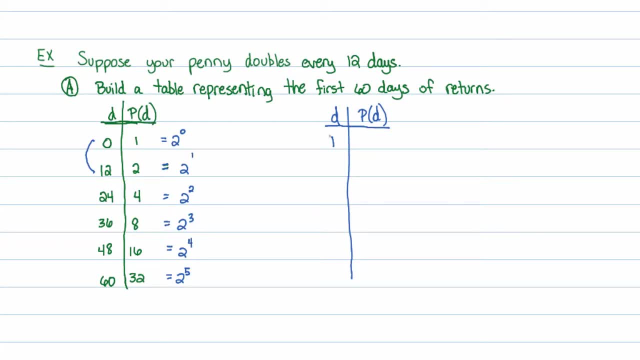 I know I have more than a penny Because It's growing And yesterday I had 1 penny, so I should have a little bit more, But it should be less than 2 pennies because that doesn't happen until I hit 12 days. 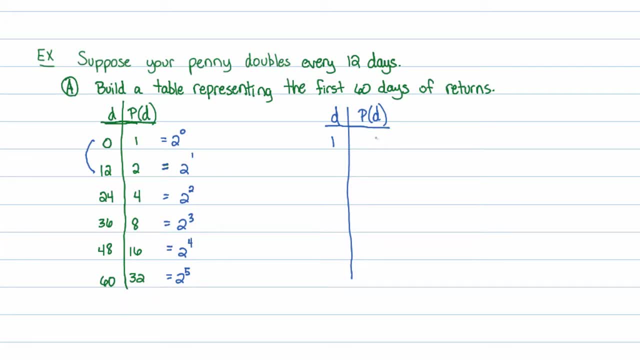 It's going to be a fractional part of that. So here's the fractional part of it: 2 to the 1 twelfth. Now the base of 2 should make sense. Everything's based on doubling, doubling, doubling. 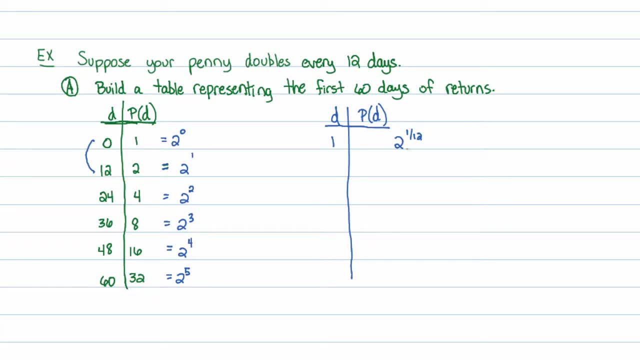 So The base of 2 should make sense, But why did I choose 1? twelfth? Well, it takes 12 days total to make the double Alright. So in other words, when day 12 comes along, I'll have 2 to the 12 over 12.. 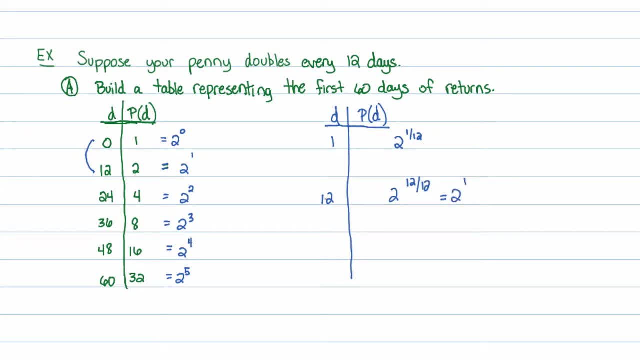 But wait, 12 over 12 is 1.. And look, that does match. It does match that right there. Well, let's see if this fractional exponent will work for 24. then 2 to the 24 over 12.. 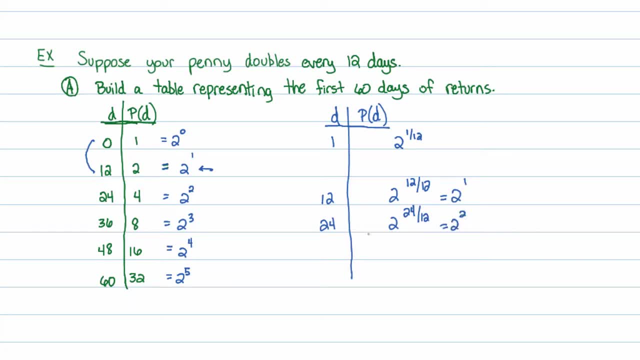 That would be 2 to the 2nd power, which is 4, which is exactly what we get. So this actually will work. Essentially, what I'm saying is if it doubles or triples or quadruples every 12 days. 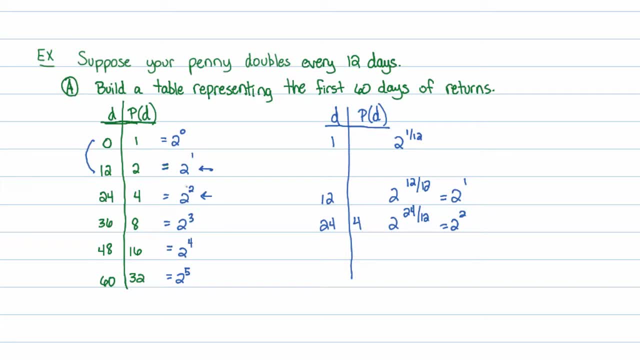 then you'll have that base for doubling, or tripling, or quadrupling 2,, 3, or 4, raised to the something over 12 power, And that something is just the number of days that passed. In fact, if you continue this on, dot, dot, dot. 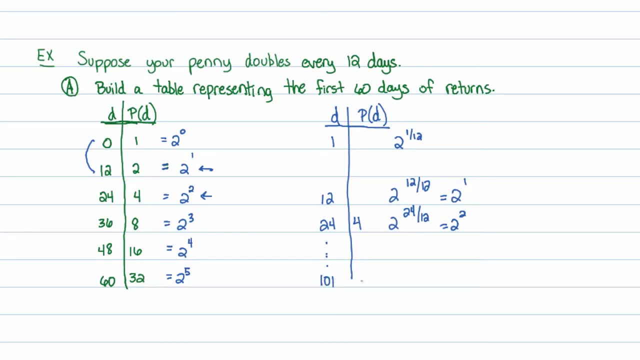 you could do like. well, after 101 days, how much do I have? Well, you'll have 2 to the 101 over 12 power, whatever that may be, And after d number of days, you'll have 2 to the d over 12 power worth of pennies. 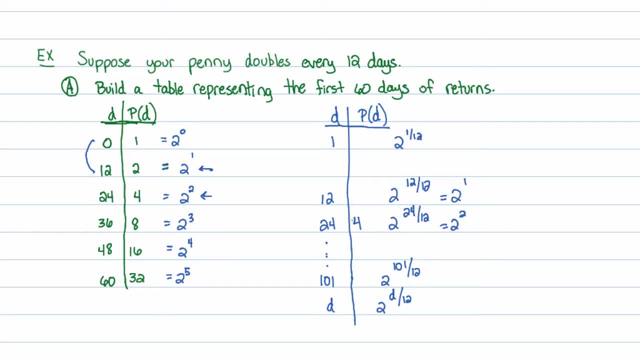 And this actually tells us the function here. So, just as a not a lot of textbooks have this supposed things double every so many days, but the fact is that's a very important skill to have, So let's go ahead and build a function for this. 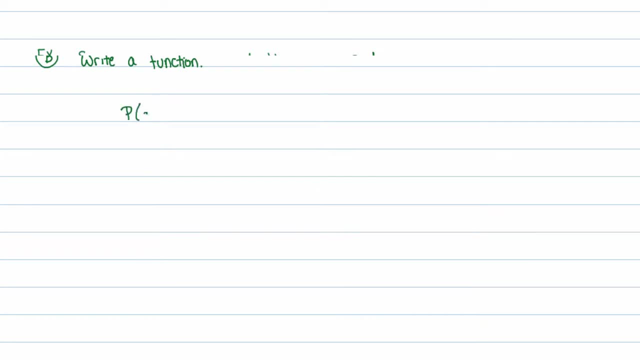 And just using the pattern from the table. actually we've already written it. P of d. the population of money that I have, depending upon the number of days I've gone by, is equal to the initial population. Maybe I should write out: it's equal to that formula, right? 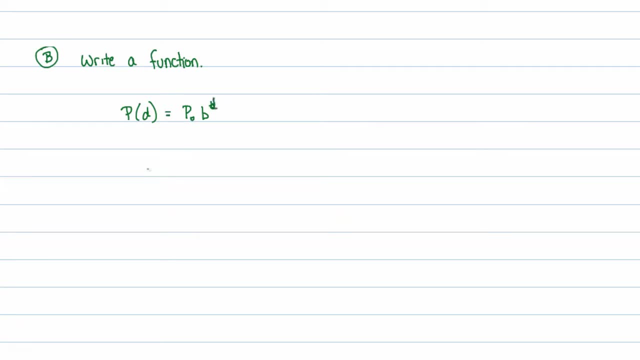 Oops, there should be a d here, not a t. Okay, So I'll just insert what I know. Initially, my population is just one penny times My growth factor is it's doubling sort of, And then it's going to be every d over 12.. 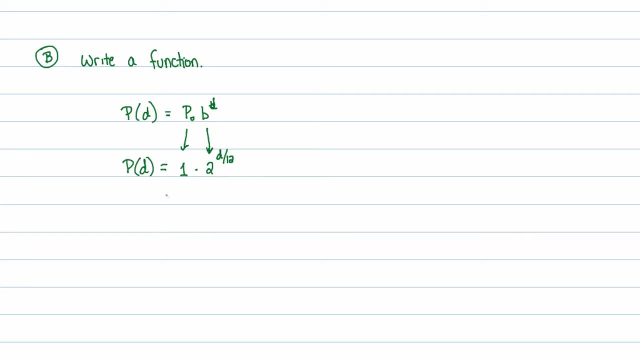 In other words, every 12 days. So let me clean this up: It's p of d is equal to 2 raised to the d over 12 power. Now there is something, There is something very interesting I should mention, or important that I should mention here. 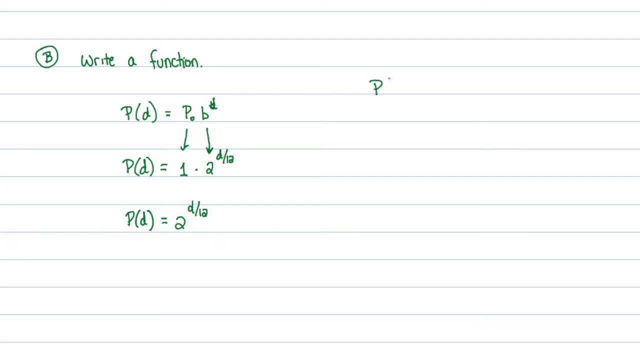 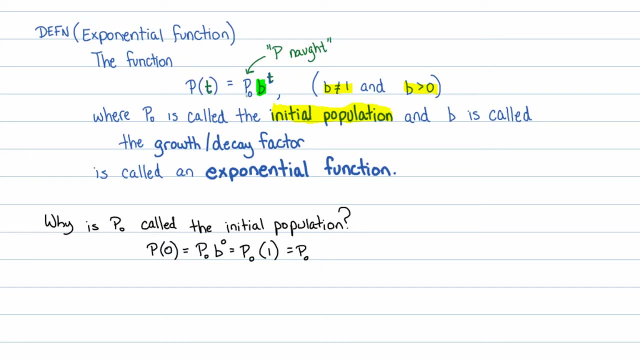 Remember that in our initial definition- actually I could just go back to it- In our initial definition here- we had this p naught times b to the t And we said that b, which is highlighted, is called the growth factor, or the growth or the decay factor. 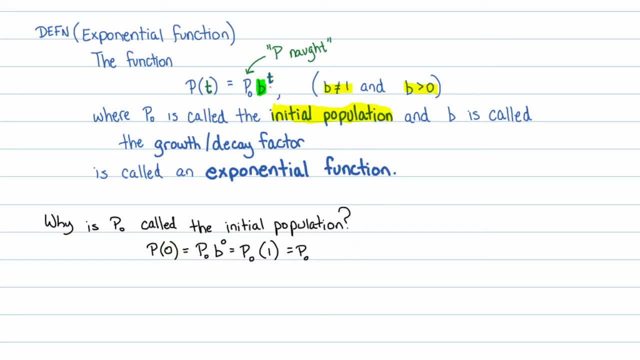 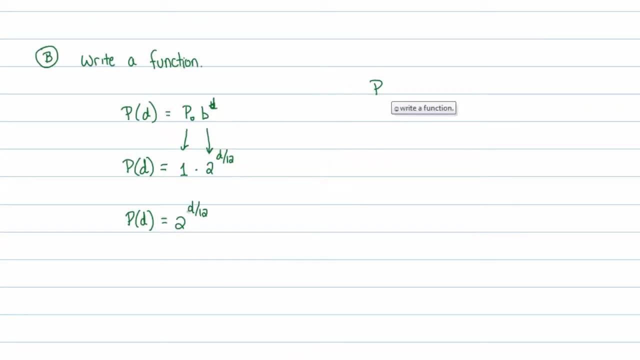 And notice the power on that is a t, Not a t over something, but a t Or a variable. So if you want to find out what the growth factor on this function really is, it's not 2.. The growth factor is kind of a manipulated version of 2.. 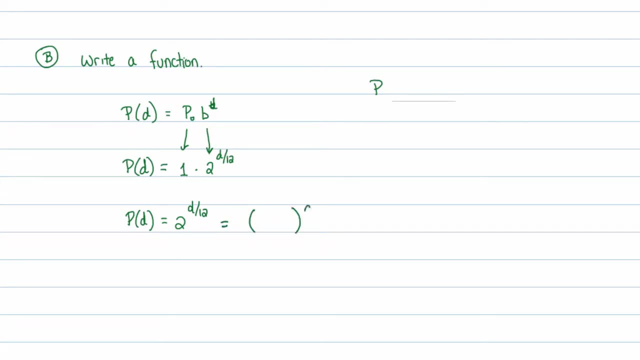 If you look at this, this is the same thing as saying something to the d power And that something is 2 to the 1 12th. Remember that's from our talk from a while ago about exponentials. If you forgot that, please go back and watch one of my videos on exponentials. 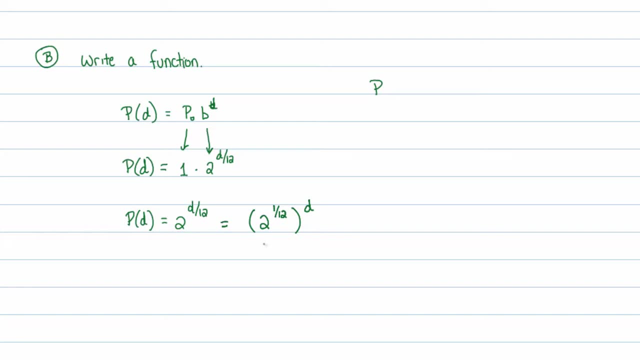 Exponential notation and that type of stuff, Powers and radicals and rational exponents, Because this is a law of exponents, that you can break that apart. Powers to powers: multiply- So now I have it in the form of p, of d, is equal to something raised to the power d. 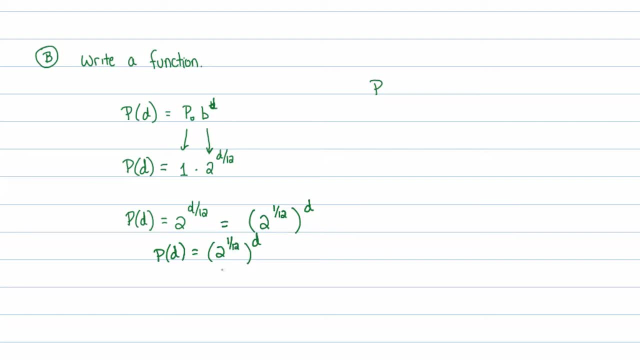 And that something is actually our growth factor, So this is called the growth Factor. It's our first time, of course, with most exponential objects, But even people who have dealt with other classes or who have taken intermediate algebra in the past probably haven't seen this. 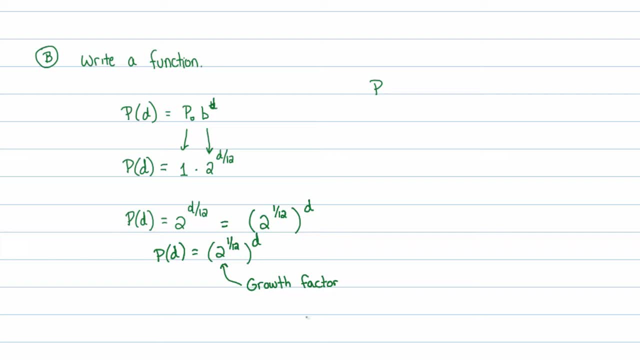 This is not something that a lot of intermediate algebra textbooks go through, But I think it's very important for you to know it. So just know that if you want to find the growth factor for an exponential function, make sure that you write the base raised to the. 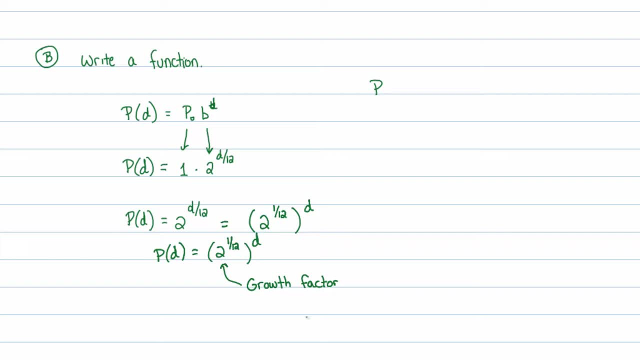 only the variable power, Not the variable over something, But basically factor out. Do this business Right From here to here, So that'll give you the growth factor. Now I can't leave this alone. I have to ask one more question. 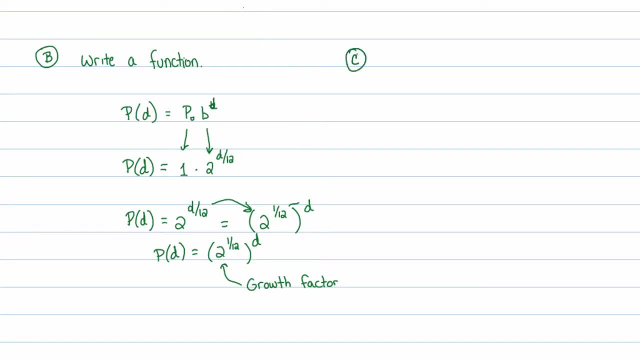 I always With exponential functions, I always do So. how much would you have after a year? How much after a year? And remember we had like $10 million after 30 days if it was doubling each day. But we're not doubling each day. 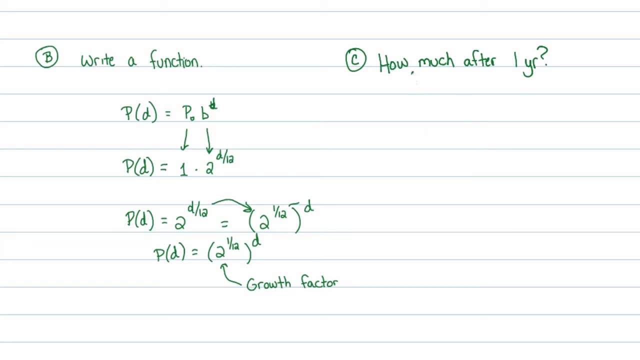 We're doubling every 12 days. So let's see how much we have after a year And let's just say that's 365 days. I know there's leap years and stuff like that, So 365 days- Plug that in. 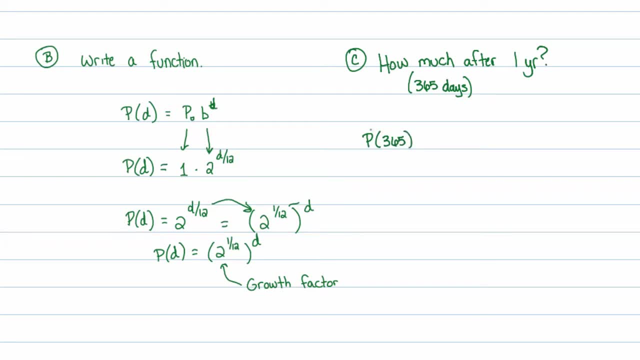 365. So we want to find out what the population of pennies is after 365 days. Well, that'll be 2 to the 1 twelfth Raised to the 365.. Now, at this point, there's a couple things you might want to try. 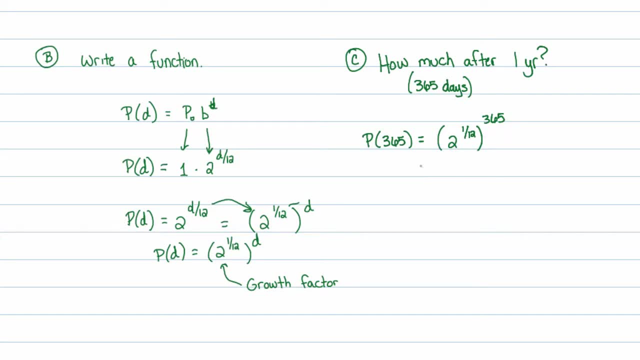 But I know it's not going to work in this case, But at this point I would probably try to do this. I'd multiply these two powers So I'd have 2 raised to the 365 over 12.. 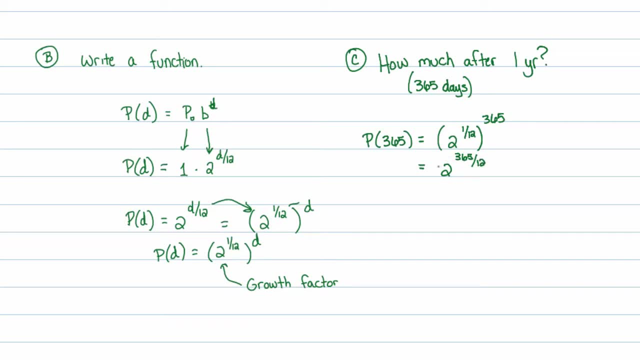 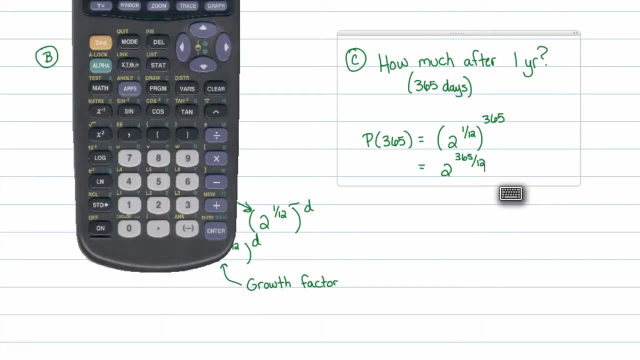 And see if that reduces. But it doesn't. I mean it only reduces slightly. So it's better to just grab a calculator. So I'll just go ahead and open up my calculator here And I will. 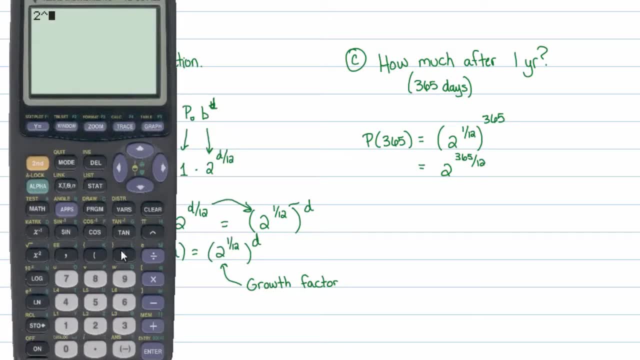 I will type in 2, raised to the Start, a parenthesis when you have an exponent like this, When you have some math in an exponent- 365 over 12. And end your parenthesis, even though it's not necessary, And you'll have this many pennies. 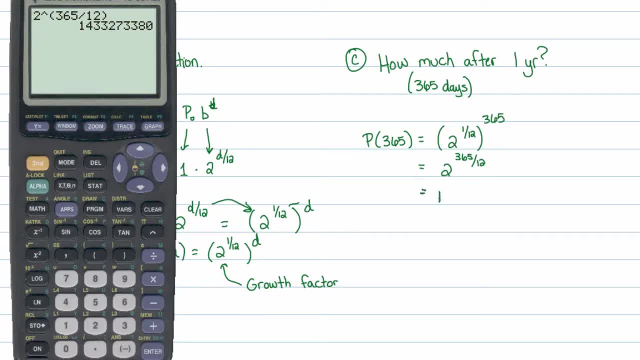 Well, we'll see how that compares. So this is equal to 14, 3, 3,, 2, 7.. What do we got? 3, 3,, 8, 0.. And again I'll convert from pennies to dollars. 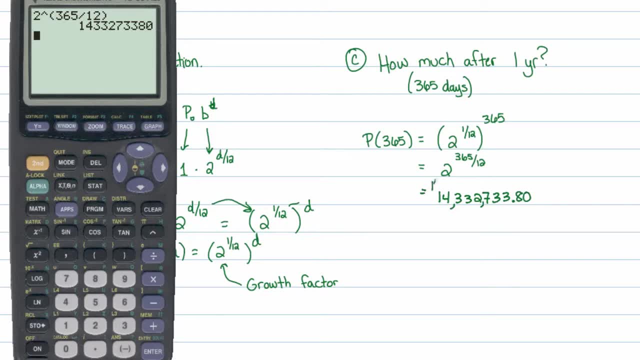 Here, put in some commas: Oh, we actually have more money. Well, of course, we had it going for much longer, But $14 million Not bad More money, but it took us 365 days to do it. 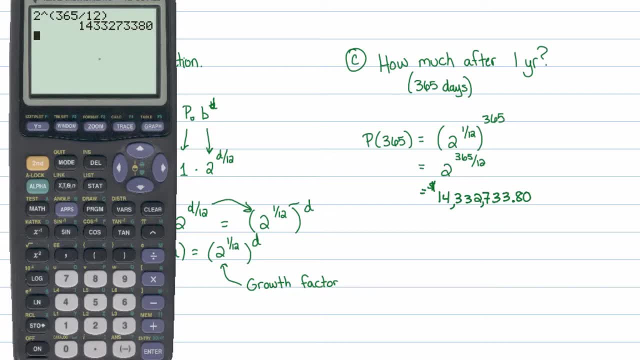 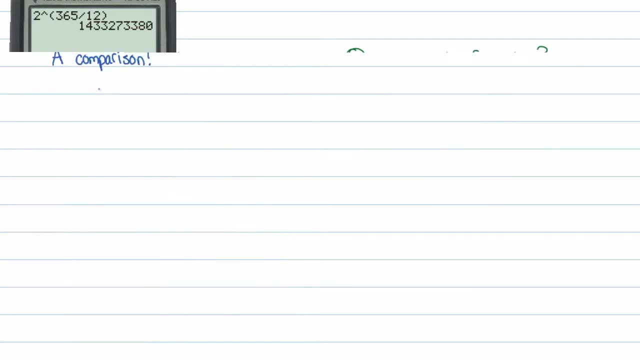 And it's more money because it was going every 12 days, But again for 365 days. Finally, I just want to draw your attention And again, this is not something that most textbooks talk about. Your textbook probably doesn't have it. 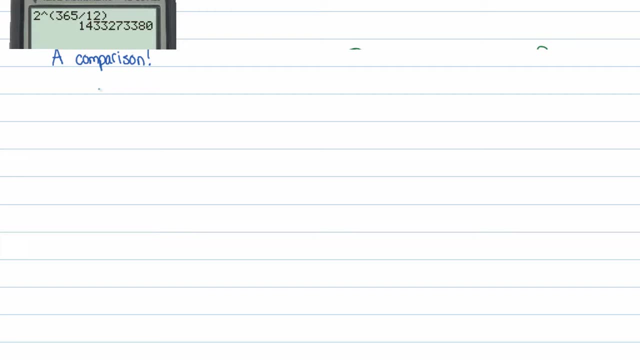 I know my textbook doesn't, But I want to compare two objects in mathematics that you have been introduced to, One being linear functions and one being- this- exponential functions, And I want to compare them and tell you that they're actually very similar to each other. 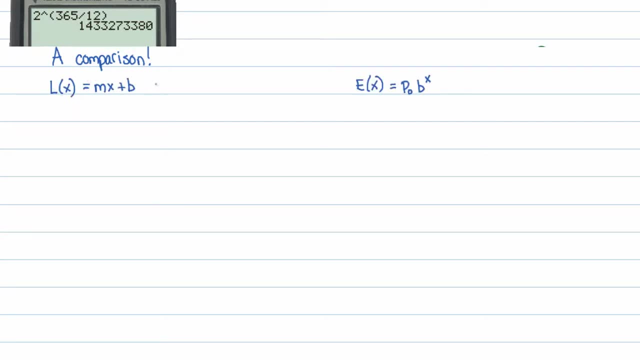 So I have a linear function right here. I'll just write that in linear: mx plus b, That's basically y equals mx plus b, right there. And this is an exponential function. And it's exponential because the unknown is in the exponent. 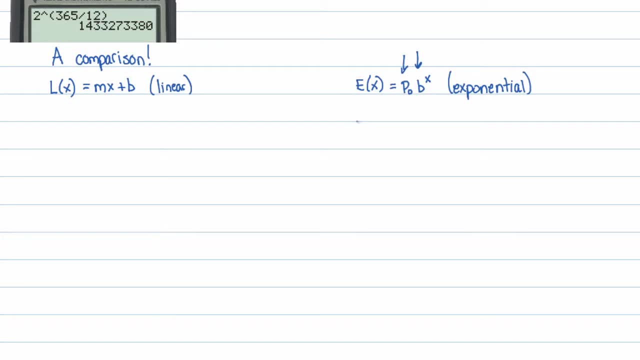 It has an initial population and a base right. There we go, But these are very similar sort of If you take a look at. Just give a simple example like this, Let's do: y is equal to 3x plus 1.. 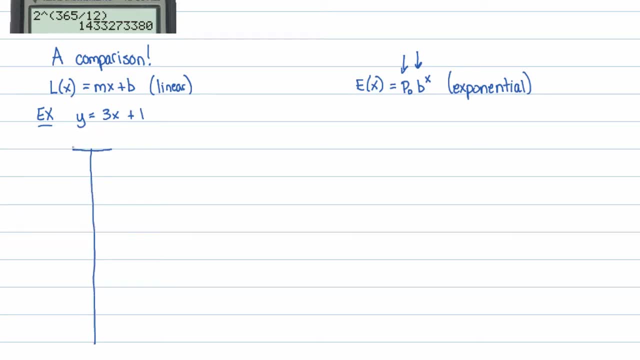 And we build a table. We have x's and y's And you know you can choose whatever you want for x's, really 0,, 1, and 2.. And let's plug in negative 2 into x here. 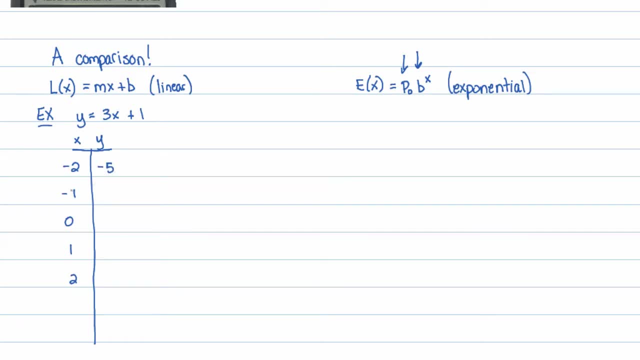 That's negative 6 plus 1.. That's a negative. 5. Plug in a negative 1 for x, You'll get a negative 3 plus 1, which is negative. 2. Plug in 0 for x, You'll get a 1.. 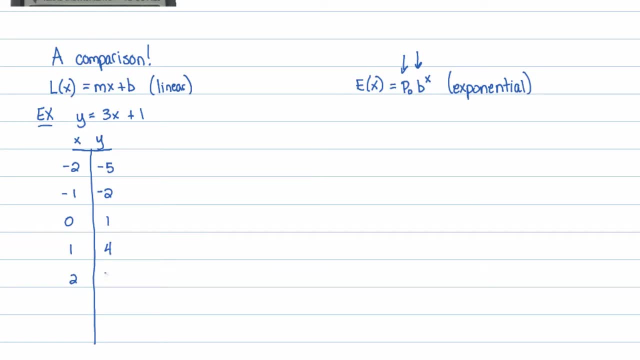 Plug in 1 for x, You'll get a 4. Plug in a 2 for x, You'll get a 7. Something you should know, you should recognize at this point, being as advanced as you are, that each step, step by 1,. 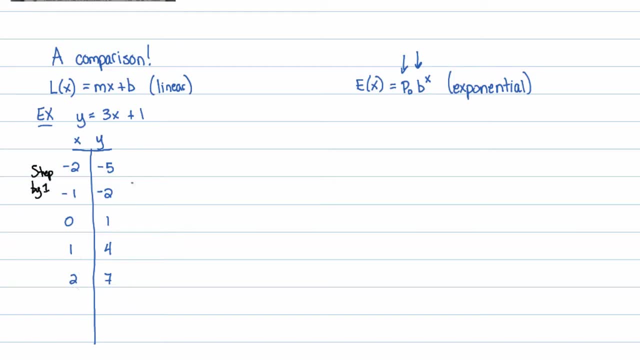 each of these x values are stepping by 1, right, Notice what the y values are changing by each time. To get from negative 5 to negative 2, it's adding 3.. To get from negative 2 to positive 1,. 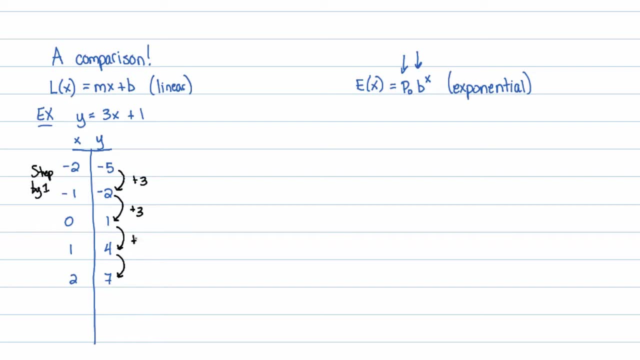 it's adding another 3.. To get from 1 to 4, it's adding another 3.. To get from 4 to 7, it's adding another 3.. So there's something this is called the slope addition property. 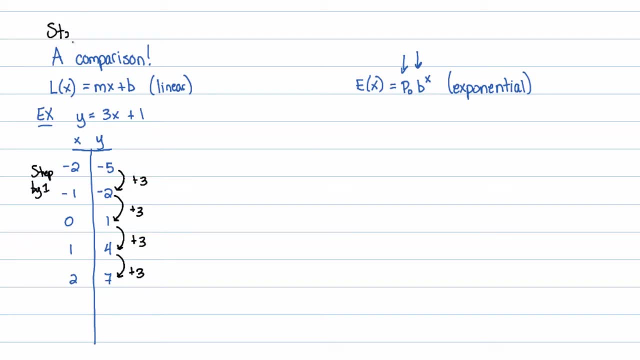 Let me write that down: Slope- Oops, that's not how you spell slope. And it basically means that if you increase x by 1, so you add 1 to x- it'll increase the y value by y by x. 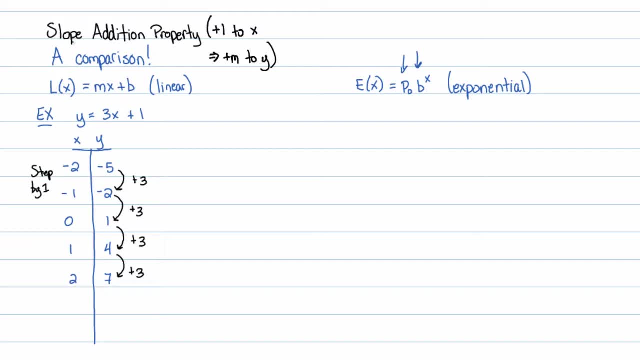 M. I'm sorry. It'll increase the y value by the slope, So you are adding the slope. That's why I call the slope addition property. Now let's take a similar example for the exponential function. So let's say, suppose that we have an exponential function. 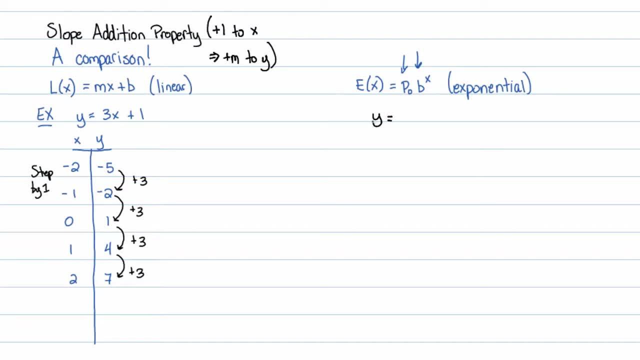 and it looks like this: Y is equal to- oh, I should use same colors- Y equals 2 times 3 to the x. Let's build a table here. Notice, let's start talking exponentially here. The initial value is 2.. 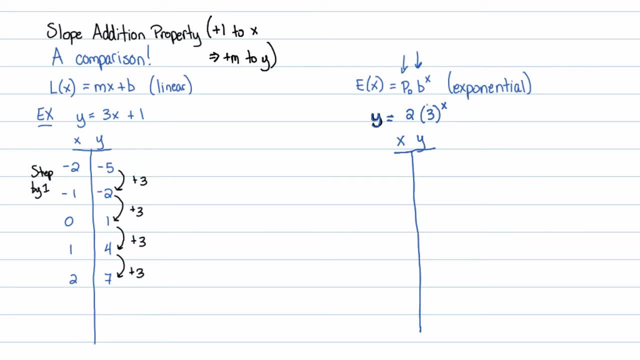 In other words, our initial population is 2.. So we have 2 objects And that 3 is the growth factor. It means it's tripling. So I start with, let's say, 2 cars and I triple every day. 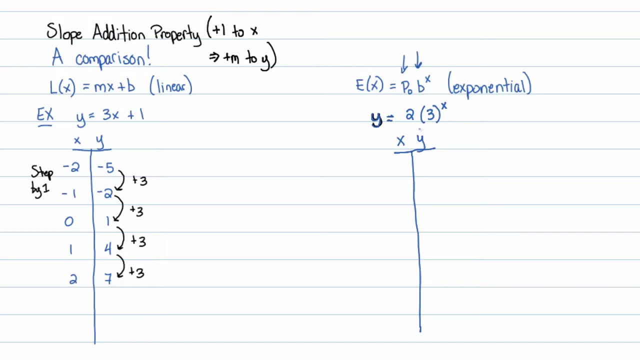 Or I start with 2 rabbits and the population triples every week, or something like that. Okay, So whenever I see an exponential function, I immediately put some situation to it that makes sense. to me, The rabbit one actually does kind of make sense. 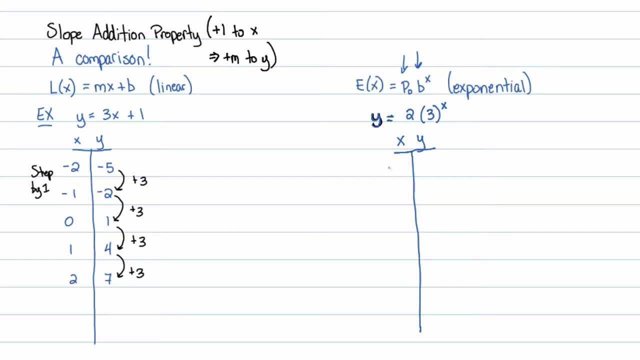 Well, no, not really All right. So let's plug in the same values for x here, Negative 2,, negative 1,, 0,, 1, and 2.. When x is a negative 2, we have 2 times 3 to the negative 2 power. 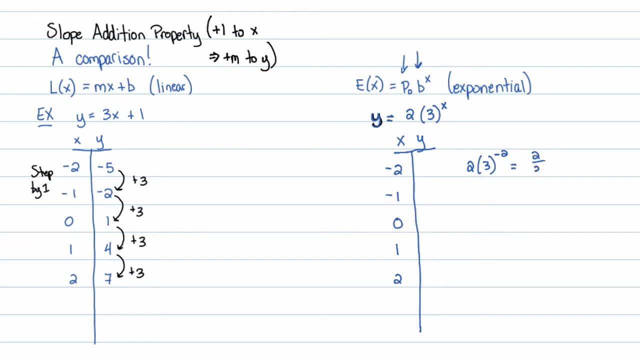 Which is actually going to be 2 over 3. squared right, You can rip the negative off and pop that downstairs And that's 2 ninths. So let me write that in there: 2 over 9.. When x is a negative, 1,. 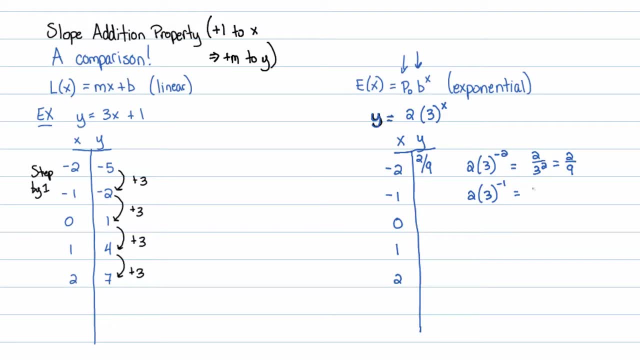 you have 2 times 3 to the negative 1. Remember, you can rip the negative off the exponent And that base of 3 will drop downstairs and the exponent will become positive. So that's just 2 thirds. 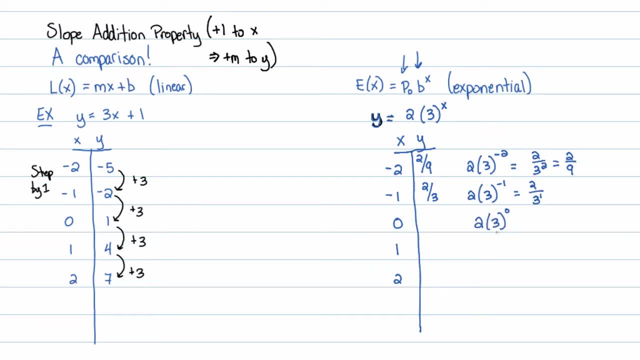 When you let x equals 0,. well, that's the initial value, And 3 to the 0th is just 1.. So it's going to be 2 here, And I could have told you that just by reading the initial part here, right? 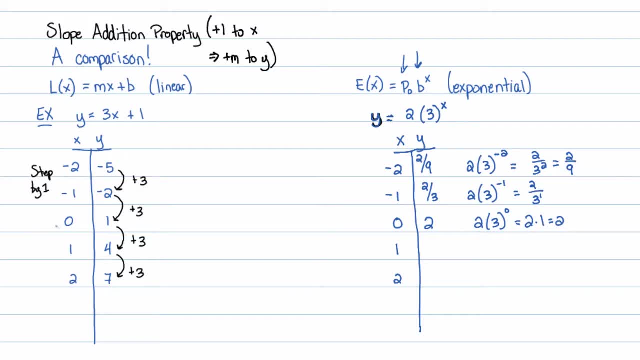 Same thing actually over with the linear function. over here, x equals 0 is the initial value, It's the y intercept, So that's my initial value there. But p naught is the initial value for an exponential function. Alright, Let's see. 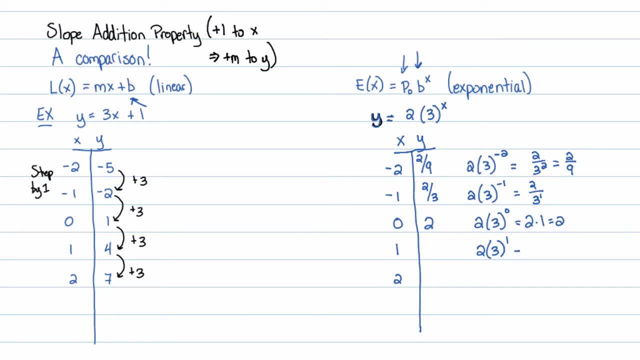 Plugging in x equals 1, we'll get 2 times 3 to the first, which is just 6.. And finally, plugging in 2.. 2 times 3 to the second power, we'll get 2 times 9 or 18.. 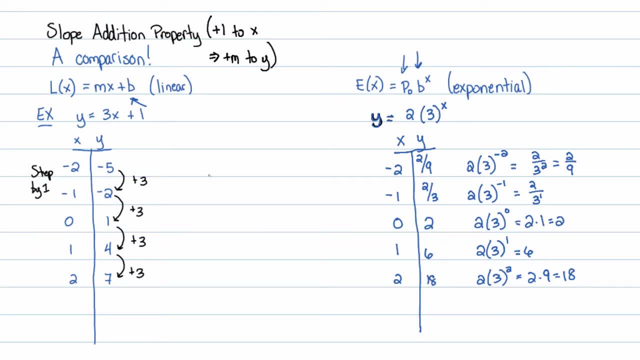 Now I told you that linear and exponential functions share something in common, or something similar in common. Notice, when I built this table on the left-hand side for my inputs, I was stepping by 1. I was just increasing the x values by 1 here. 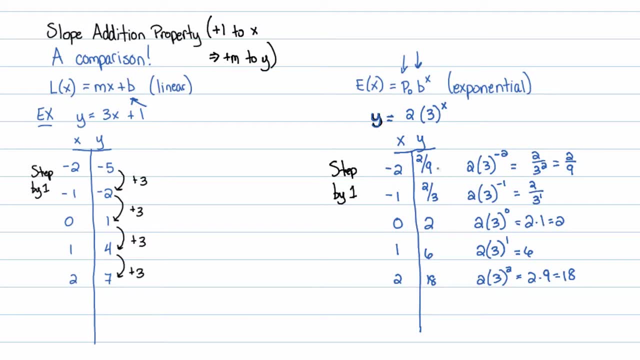 You can continue building the table if you want. And something happened with the outputs. Each of these outputs did they increase by the same amount every single time. Did we add? like to get from 2 to 6, we added 4.. 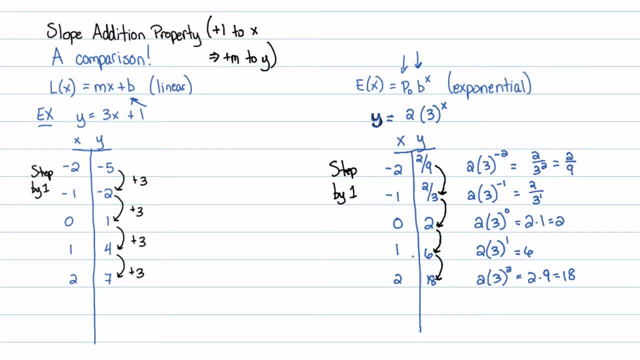 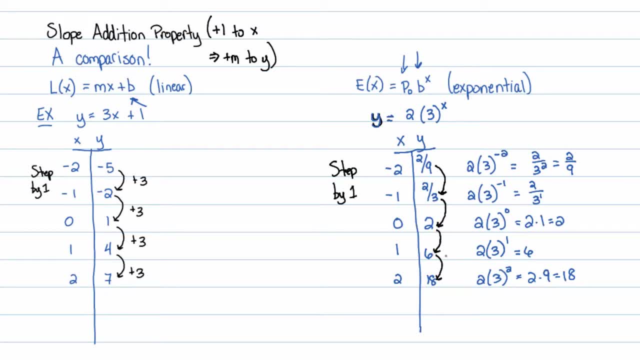 But notice that to get from 6 to 18,, you would multiply by 3.. To get from 2 to 6, you would multiply by 3.. To actually get from 2 thirds to 2, you would multiply 2 thirds by 3.. 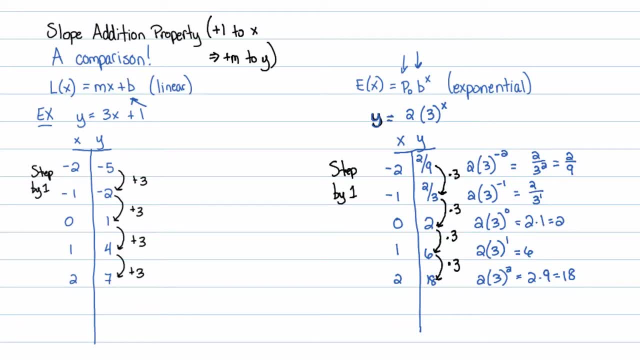 To get from 2 ninths to 2 thirds, you would multiply by 3.. Now notice how similar these table setups are, This idea that every unit is equal to the output, and every step in the x direction. you multiply the output, the y value, by the base. 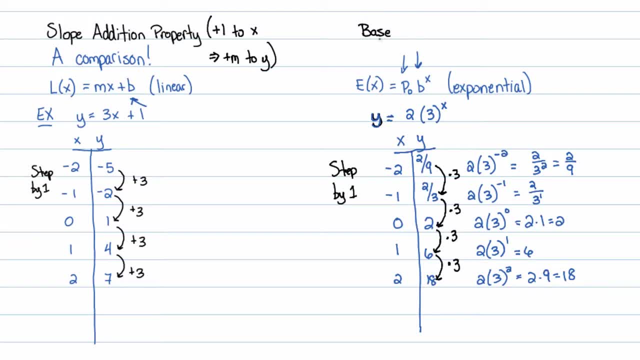 is called the base multiplier property, Which basically means every time you add 1 to your x value, your y value gets multiplied by the base. That's the base multiplier property. Now, again, this is supposed to be. it didn't really work out that way. 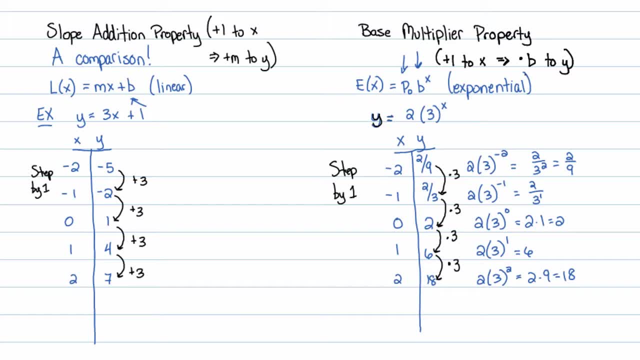 it was supposed to be the conceptual lecture, which is the idea of an exponential, you know. But I want you to know that I'm going to repeat a lot of this stuff, not definitions. I'm not going to sit there and say, oh remember.